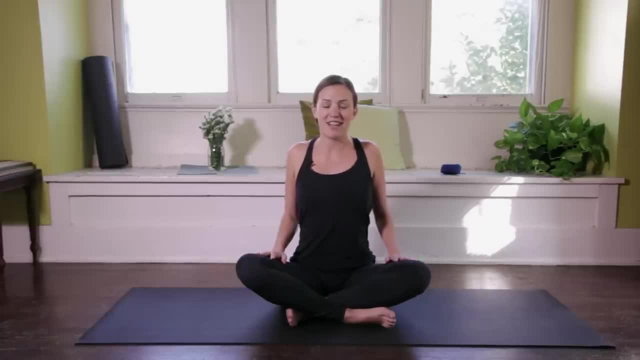 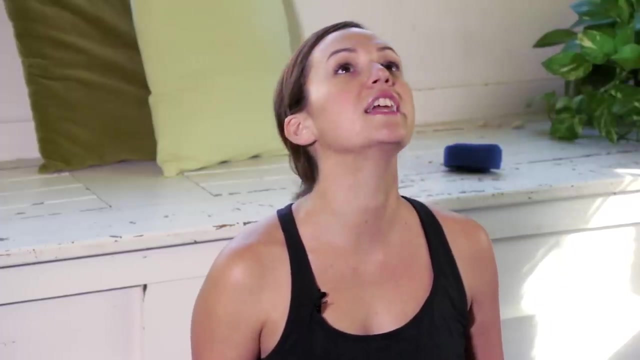 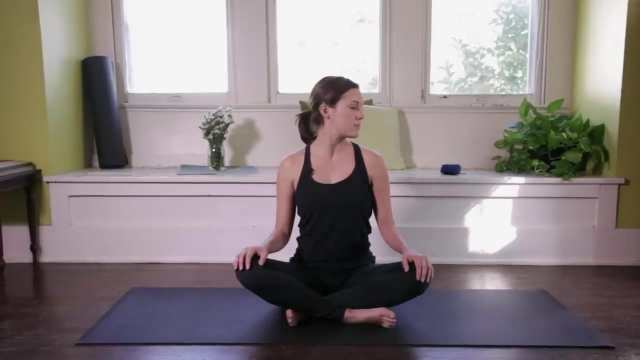 looping forward, Exhale, grounding, down and back, Just finding a little organic movement here And then maybe checking in with the neck by just maybe moving one ear over one shoulder, And then we'll go forward to the chest, Shaking the head, yes, And now no, Okay. coming back to center, we'll bring the head over the heart. 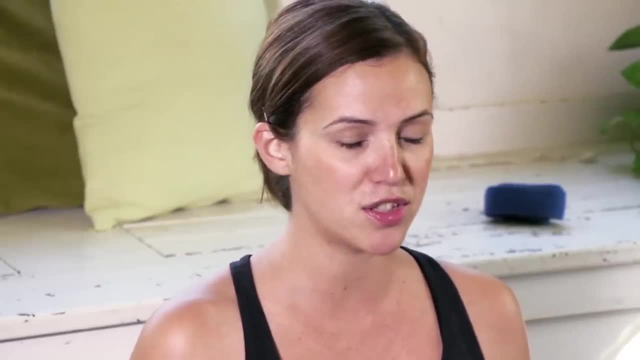 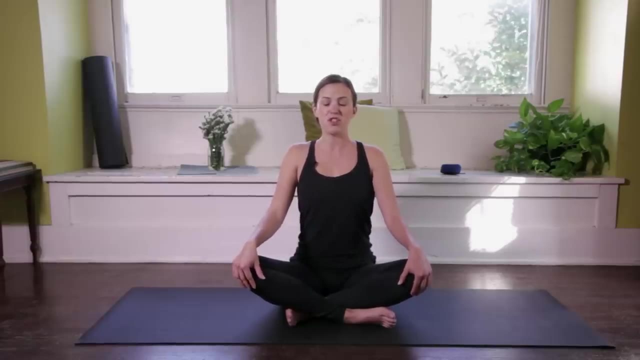 the heart over the pelvis. Okay, So take a second to maybe close your eyes or soften the gaze so you can just go inward a little bit here As we find alignment. head over heart, heart over pelvis. we lift the sternum, lift the chest and then again ground down through the elbows here on the exhale. 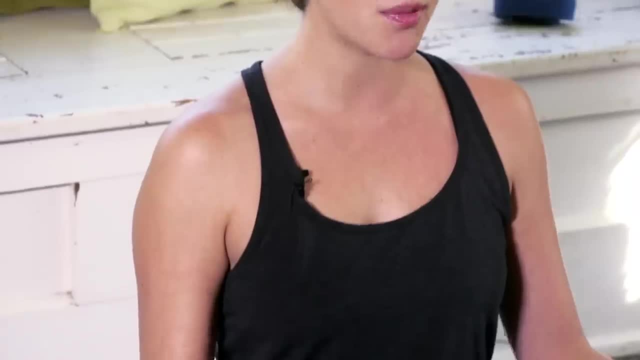 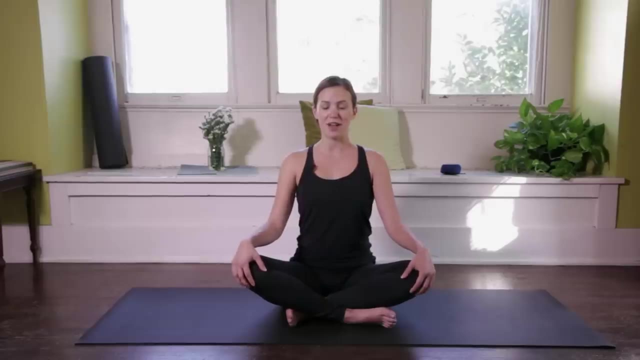 Find a nice space between the ears and the shoulders and we just kind of come into the moment with a little integrity. whatever that means to you, For me it means body awareness, mind awareness, noticing where my thoughts are and coming back to that body awareness. 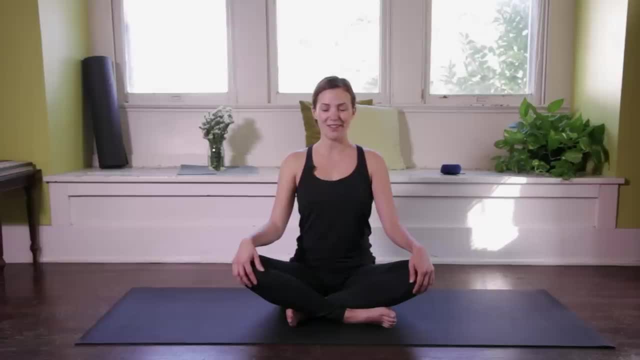 And then see if you can begin to deepen your breath here. Nice long inhale in and a nice long, juicy exhale out. Keep that going. Nice long inhalation and a nice long, extended exhale out. Draw your palms together at the heart. Take a deep breath in Each time we come here. 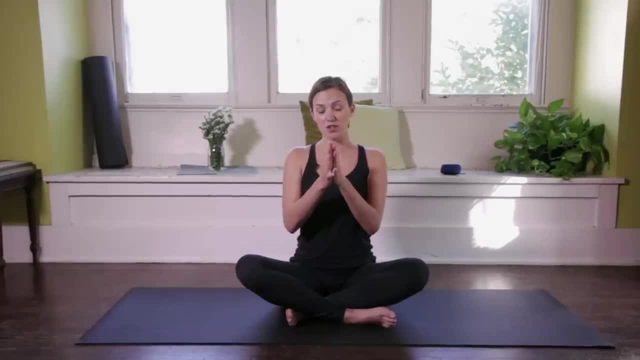 this is a great little beginner's tip. Each time we come to this mudra, we call it Anjali Mudra. you can think about lifting your sternum or your heart up to your chest. So often when we get a little bit tired- and we will in our practice- we can have this little reminder. 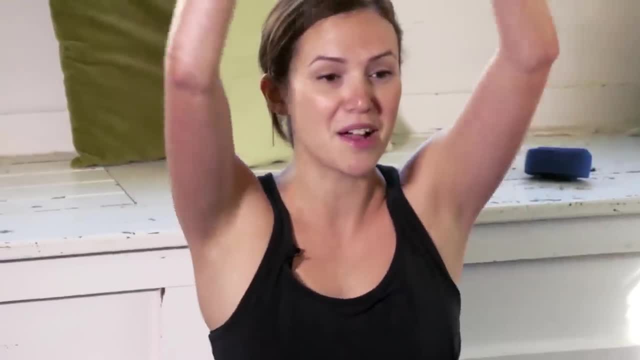 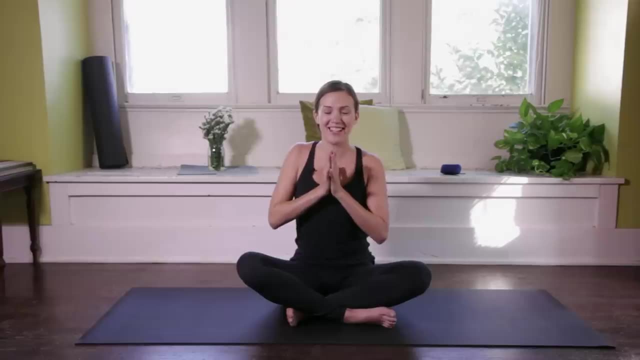 to loop the shoulders and lift the sternum to the thumbs each time we come to this hands at the heart or this prayer position: Anjali Mudra. So practice that now. Inhale, lift your sternum up to your thumbs, Draw your lower belly or. 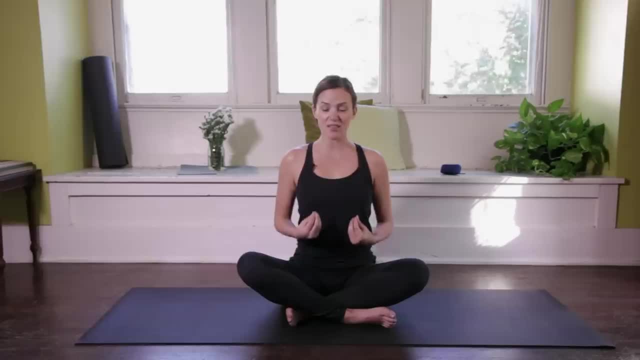 navel in to meet your spine. So again, we're just coming into this active body, but with a sense of ease. This is going to be a wonderful tool for beginning a yoga practice, just kind of finding the balance between active body, strength, engaging qualities and then also a softness. 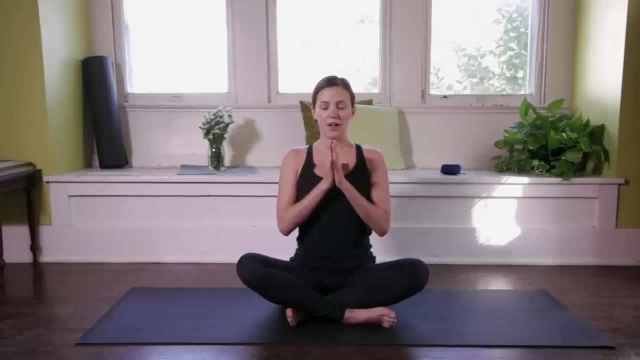 an ease, a lightness, a calmness, if you will. Finding a place where those two can dance and be together is what our yoga is all about. Interlace the fingertips, Follow your breath as you inhale, Press the palms forward up. 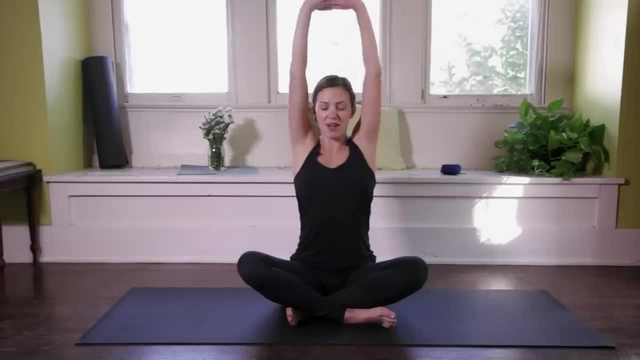 and back Nice and easy here as we climb up the side body, climb up the spine and on your next exhale release the fingertips down. Nothing fancy here, Just checking with the body, checking in with the breath inhale again. 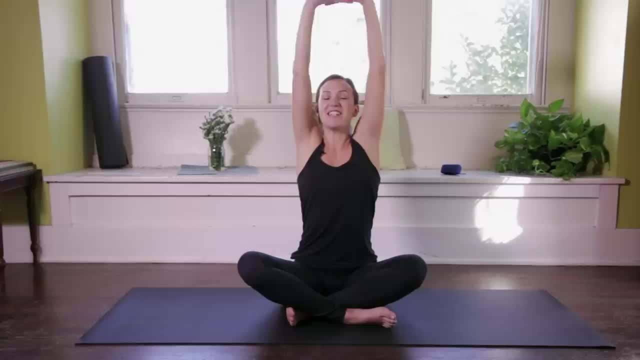 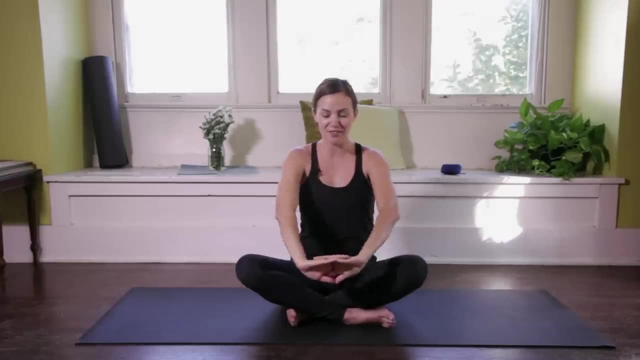 forward, up and back On your exhale fingertips release with elegance, with ease, opening the shoulders, opening the chest, checking in with the side body. One more here, as we ground down through the tops of the thighs, Deep breath and exhale. 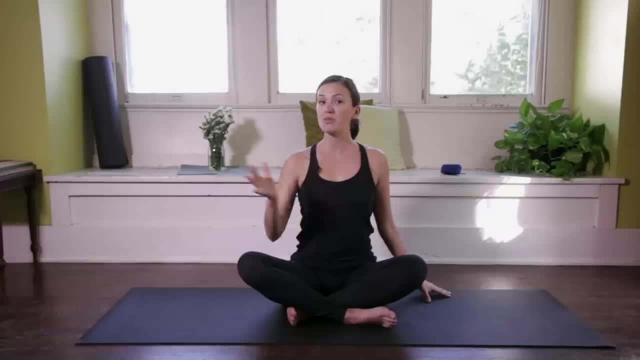 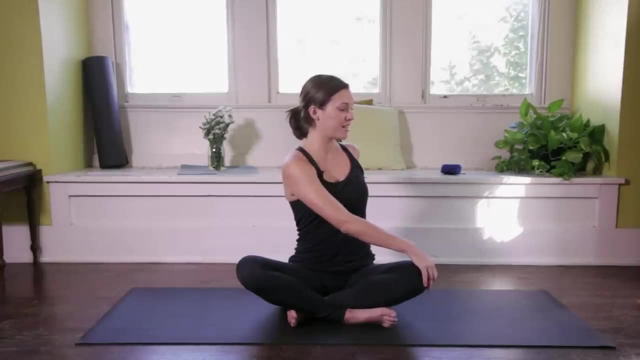 release Great. Take your right palm to your left knee, Sit up nice and tall. Send your left fingertips behind the tailbone here As you inhale, lift up, Lift your heart, Exhale, journey towards the left. Find a gentle twist here. 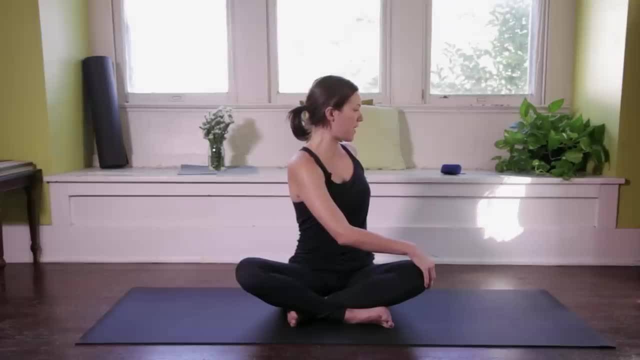 Navel draws in towards the spine And we remember that we come to the mat to have an experience in our body, So don't crank yourself into the posture. Have the experience of gently moving into the twist, Maybe closing the eyes here for one last breath. 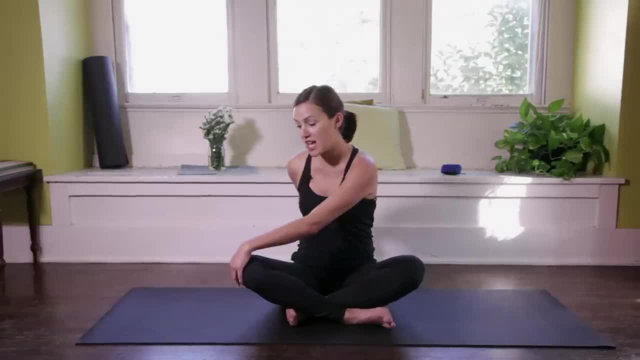 We gently release back to center and take it to the other side. Left palm to right knee. Sit up nice and tall. This time I'm going to turn to the side so you can see my spine. here The tendency is going to be to round forward. 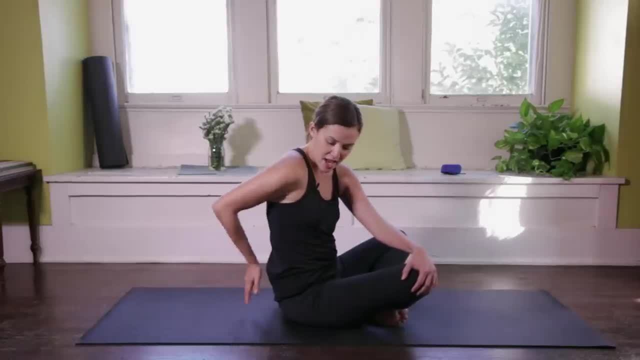 We spend a lot of time here all the time, okay, So no worries, And in time we're going to begin to lengthen Tailbone down. Lower back becomes nice and long, Heart lifts, Shoulder blades ground down and we find our twist. 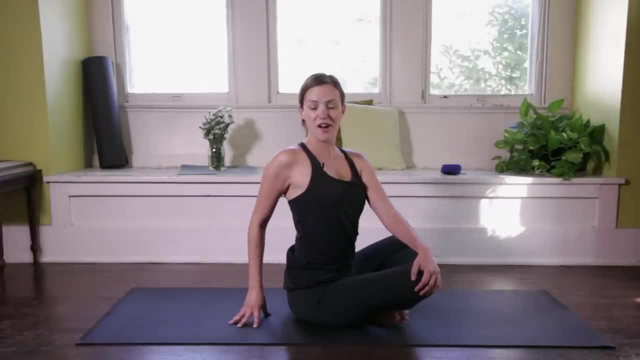 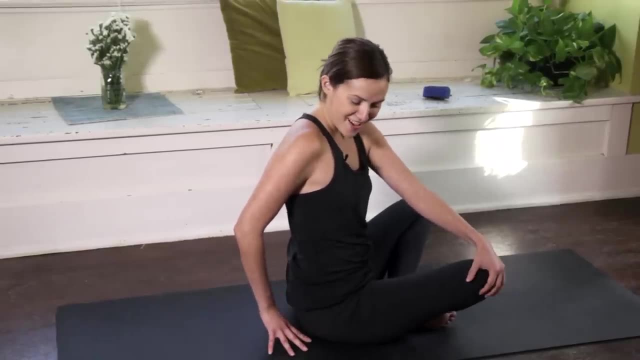 So what I'm trying to say here is: don't sacrifice this lift in the heart and this length in the spine for a deeper twist. Ouch, This is just Ouch. This is wrong. y'all This is wrong. So find what feels right, what feels good. 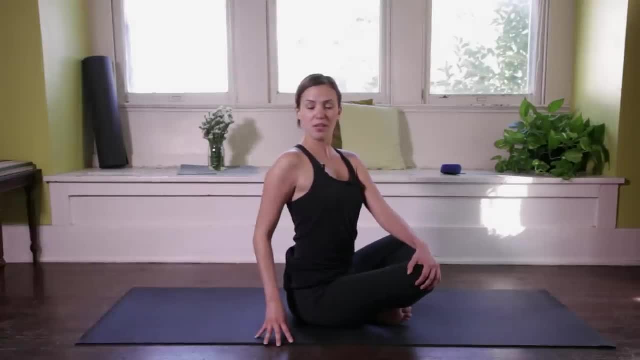 So it might mean that you don't go all the way far back at first, but keep a nice mindful twist here, Using that exhale to journey a little deeper, Even if it's just energetically, And then gently releasing back to center. 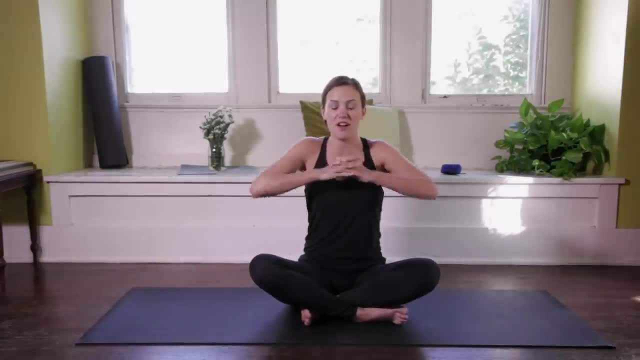 Great, Take a second here, one more time to interlace the fingertips of the heart, Inhale Palms, reach forward, up and back. Long puppy belly We stretch here, Lift it up high And then exhale, Release fingertips to the mat. 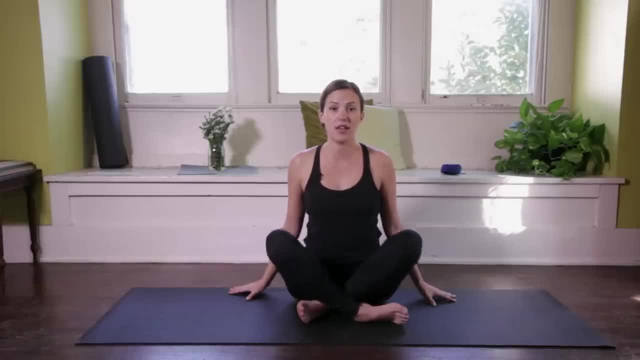 Side body stretch: Nice and easy. Keep grounding through the legs here, so the legs aren't just limp here, They're nice and active. Tops of the thighs: drawing down Great Plant your left palm or left fingertips, Yogi's choice. 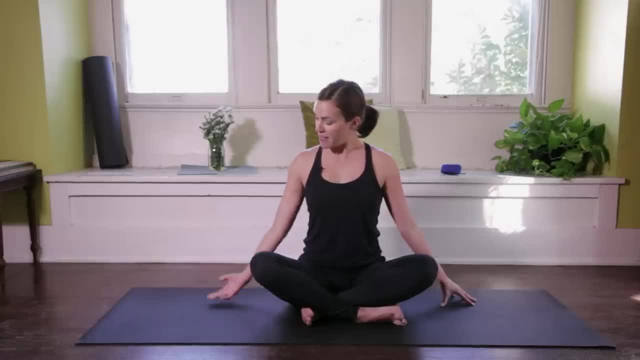 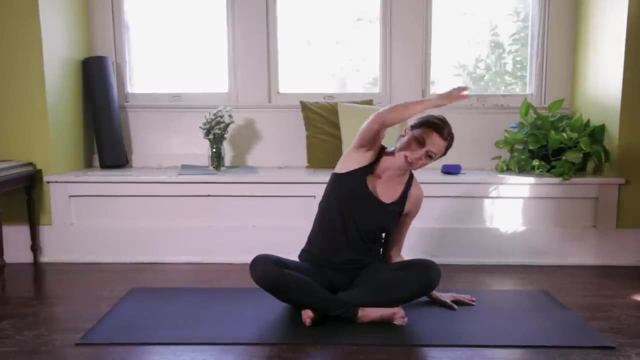 Beginner's yogi's choice. So press into the palms or the fingertips And then send the right fingertips up, Think, up, up, up up And then go over, Careful not to just go over Trying to mimic an asana that you may have seen before. 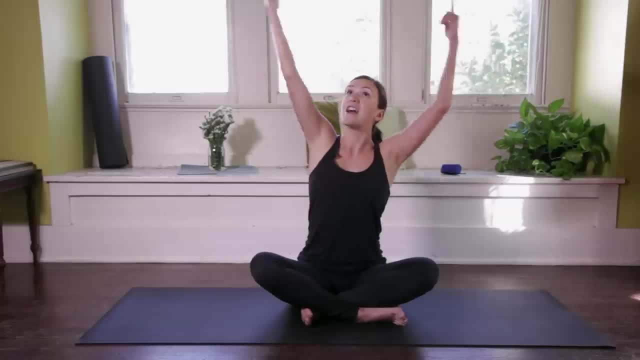 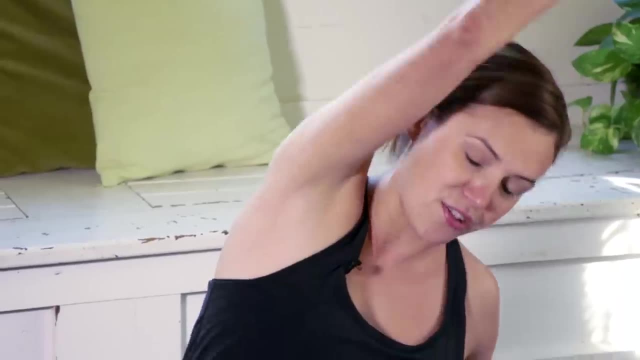 Have an experience: Inhale, Reach it up, Keep this lift in the heart And then exhale, Side body stretch. Now here we're not going to hold, but we're going to kind of set the tone for our yoga practice and our yoga journey by finding a little self-expression. 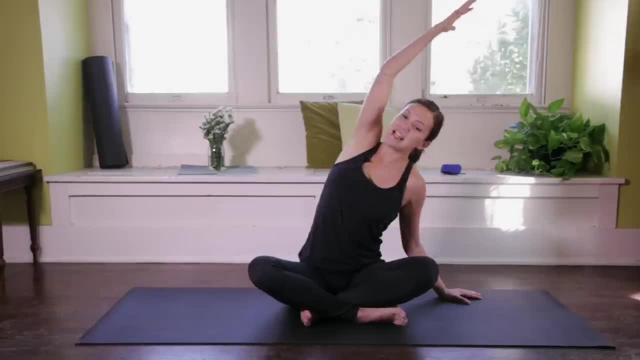 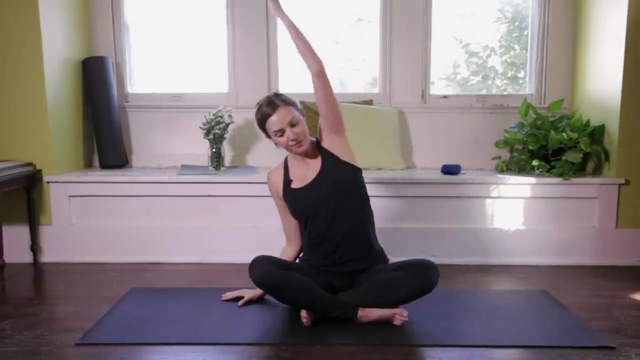 Okay, Finding a little movement here. You might sway up and down, front and back, You might close your eyes. You might stretch your mouth, You might wiggle the fingertips, Draw the shoulders away from the ears, Take a deep breath in and exhale swiftly through center and to the other side. 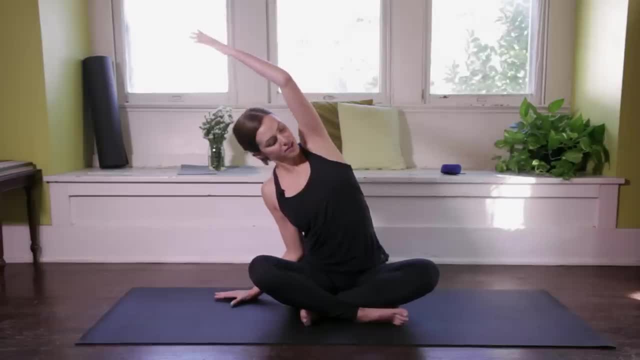 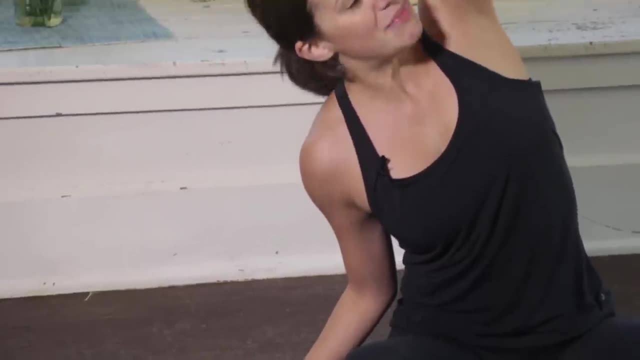 Creating space in the body, Connecting to the breath. Remember, there's no right or wrong here. It's great. It just kind of takes the edge off. We're going to learn some basics, We're going to focus on alignment, But remember, there's no right or wrong here. 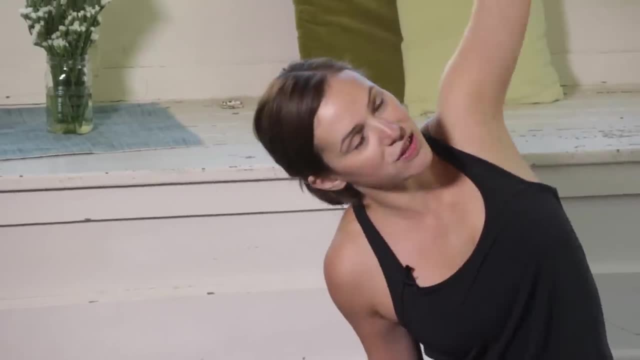 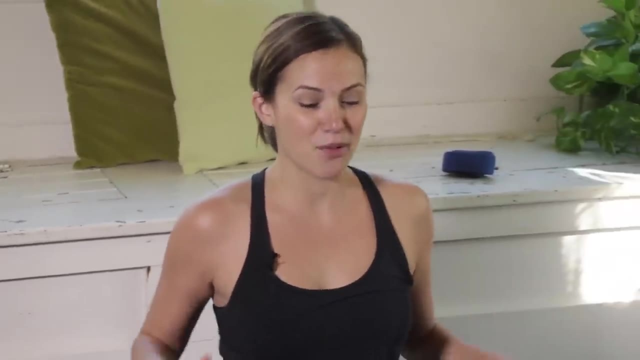 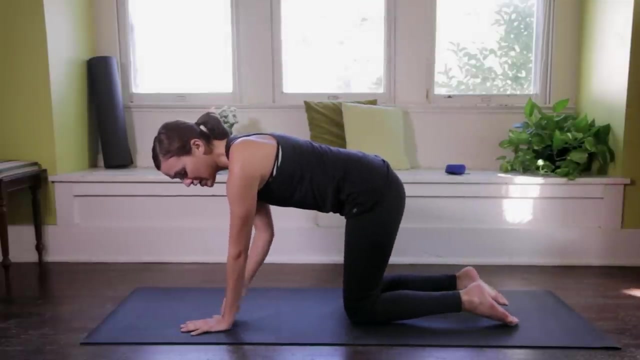 Really it's about that self-expression. So find a moment or two here to find a little movement And then, swiftly, we come back to center and we're going to take the palms and dive forward onto all fours. Okay, So I'm going to align wrists underneath the shoulders and knees directly underneath the. 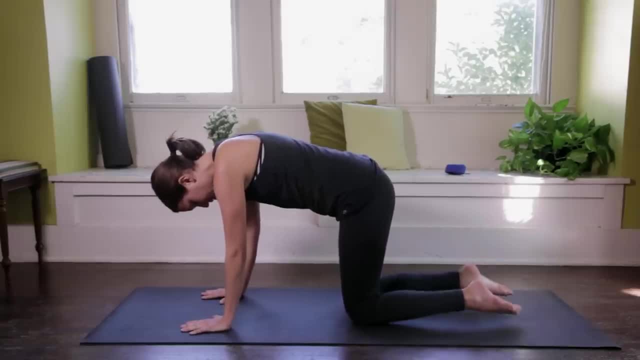 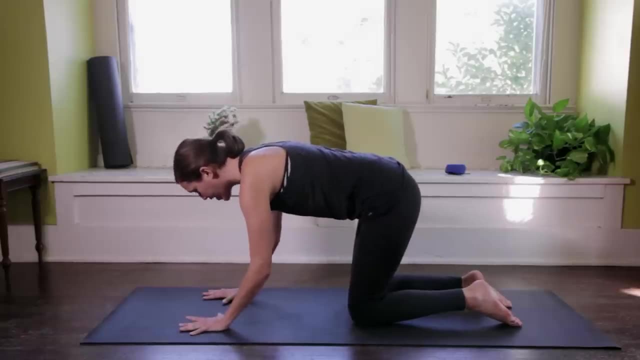 hip points. I'm pressing into the tops of my feet here, Toes are pointing straight back And my palms are spread super wide, my friends, Super-duper wide, Spreading the palms like starfish. Now, the most important thing I can teach you at this moment is to connect with this upward. 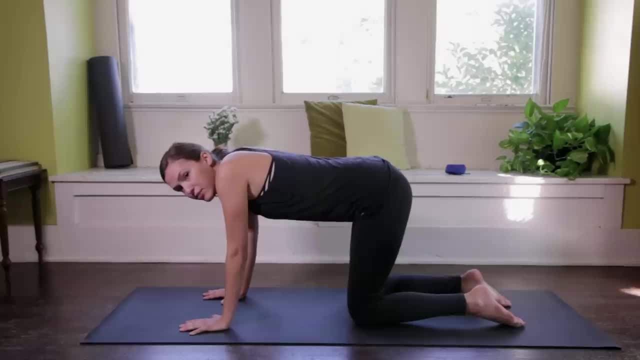 current of energy, whatever this means to you. And that means not collapsing into the bones here, but pressing up and out of the earth. Okay, So that means connecting to every part of the foundation, all parts of the body, that's pressing into the mat. 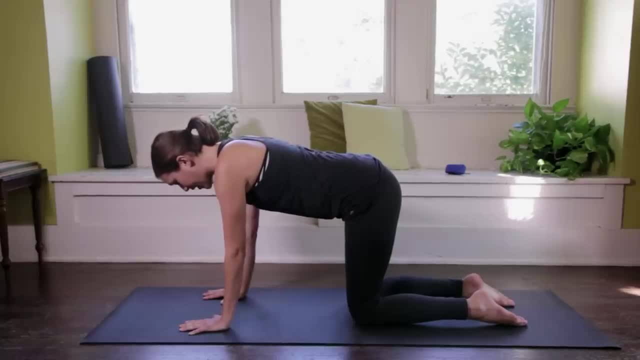 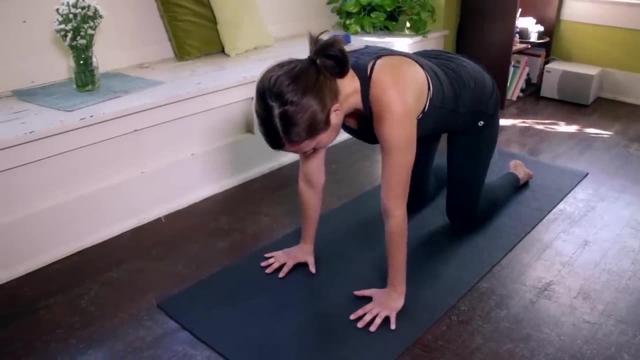 And then remembering to find that integrity- head in the heart, heart over the pelvis- but maybe creating a nice tabletop position here So we're not sitting up straight anymore. We've moved our center of gravity, But I can still work with that alignment: head, heart and pelvis in line. 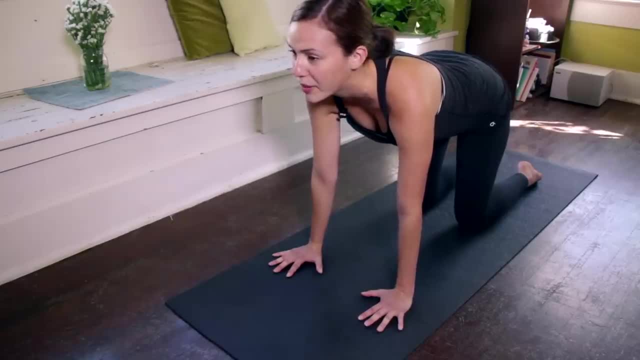 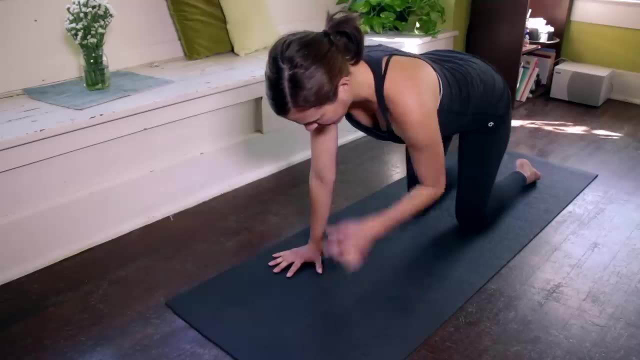 Notice how I'm drawing my shoulders away from the ears And I'm remembering that my head, this neck, is an extension of the spine. So I'm not hanging out here, I'm not crunching here, But I'm going ahead and taking the gaze down for now and finding a nice long, beautiful. 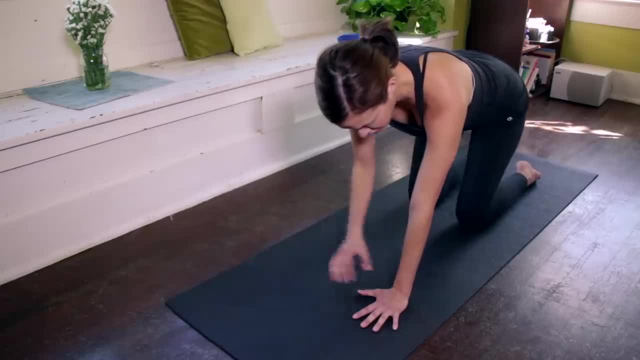 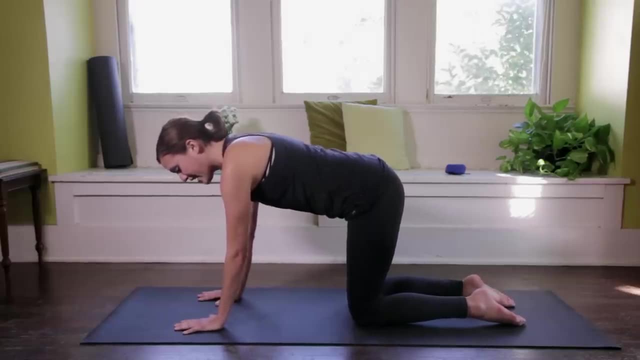 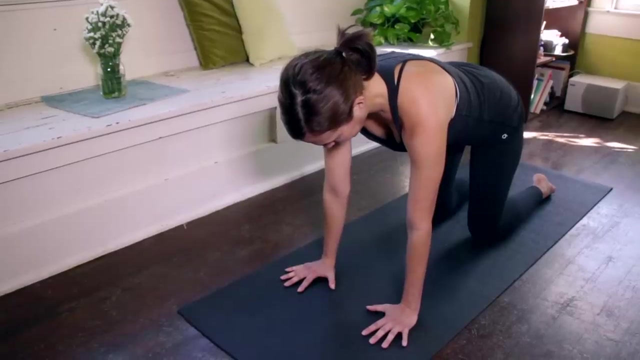 neck. Great, You might feel a little bit of pressure in the arms and the wrists here. Keep pressing up and out of the palms So that we can begin to build strength rather than collapse into the bones. Okay, From here one more breath. I'm going to exhale. 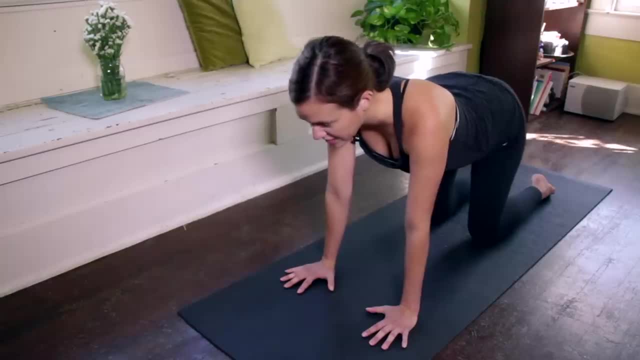 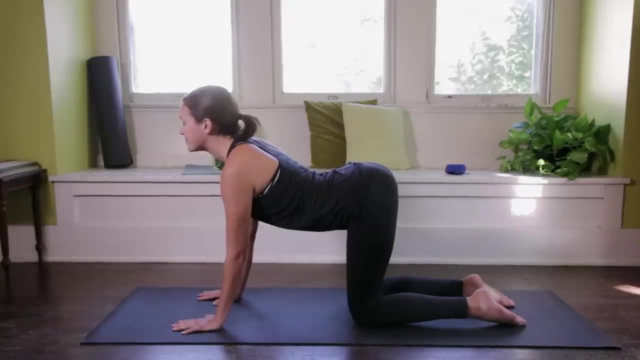 On your next inhale loop. the shoulders drop, the belly Tailbone tilts up towards the sky as I look forward. Little cat-cow here, Long neck, Take your time. No rush On the exhale. I start at my tailbone. 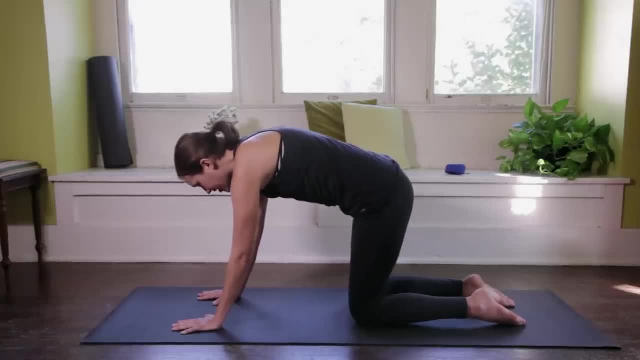 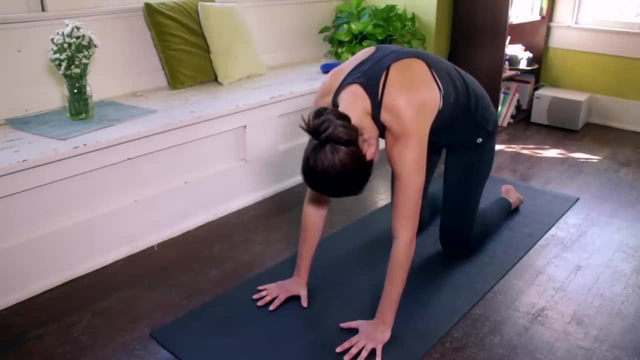 I travel up the spine, Drawing up the spine until the crown of the head is the last thing to release. Take a breath cycle here, In and out, Letting the weight of the head go Navels, drawing up towards the spine And pressing into the tops of the feet here. 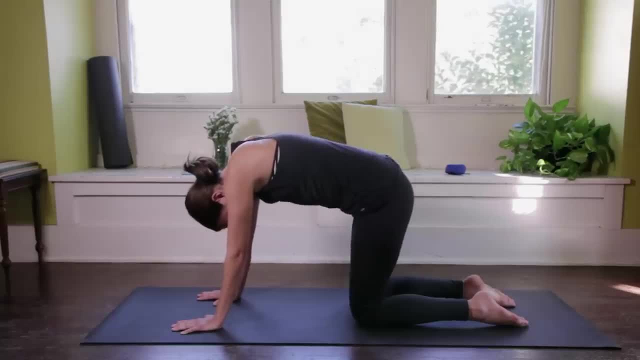 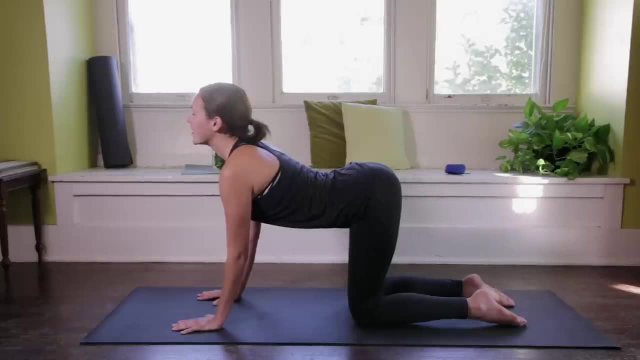 I'm pressing up and out of the palms, Deep breath in Inhale, Looping the shoulders. Heart radiates forward. Then on the exhale, tucking the tail, Drawing the navel up, Closing the eyes To really have an experience. 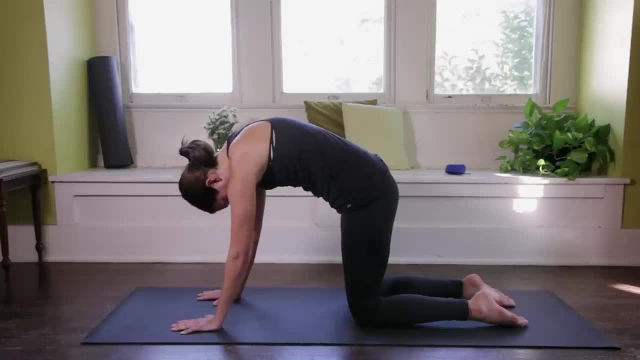 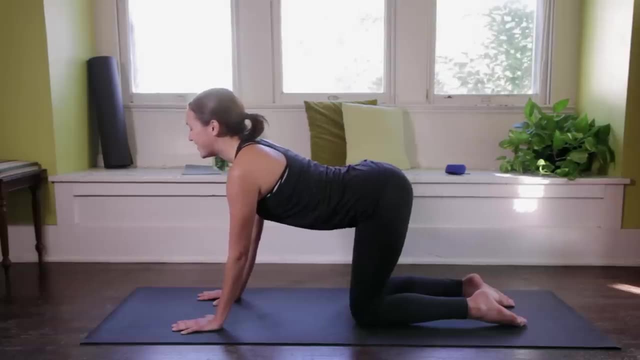 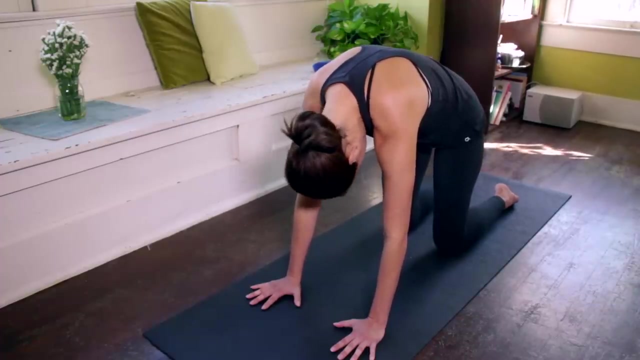 We call this spinal flex or cat-cow. And one more Inhale, Pressing into all ten knuckles, Exhale, Curling the tailbone in Starting there, Traveling up the spine Chin to chest Crown of the head, releases. 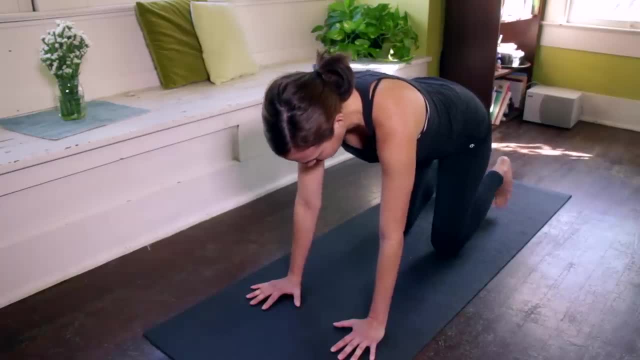 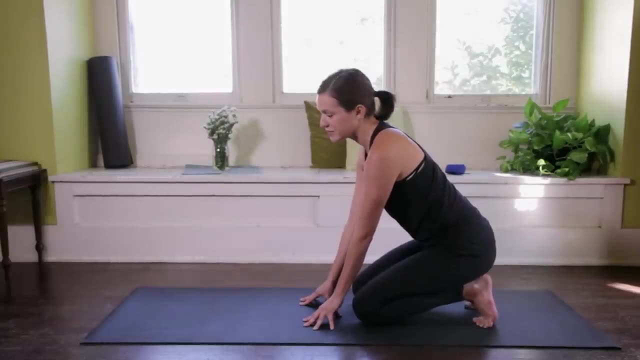 And then we inhale back to tabletop position. Curl your toes, Walk your fingertips back. A little yoga for the feet, Little beginner's feet moment here. So for some this is no biggie. No biggie For others: your feet are. 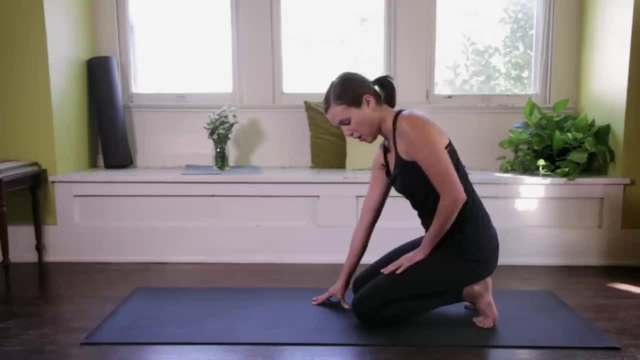 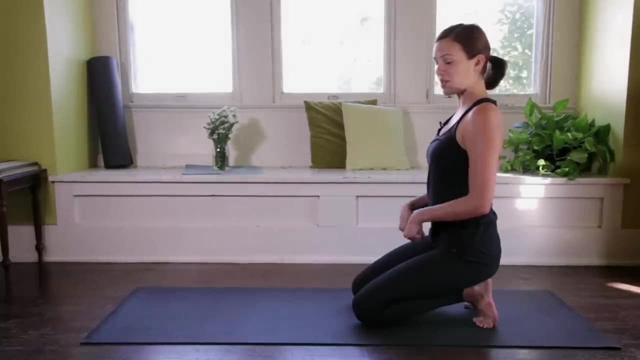 Your dogs are barking at you right now, So you might just stay here. Others might walk the palms all the way up. Find that lift in the heart. Deep breath in Press into your pinky toes. This is a great opportunity to roll the wrists out. 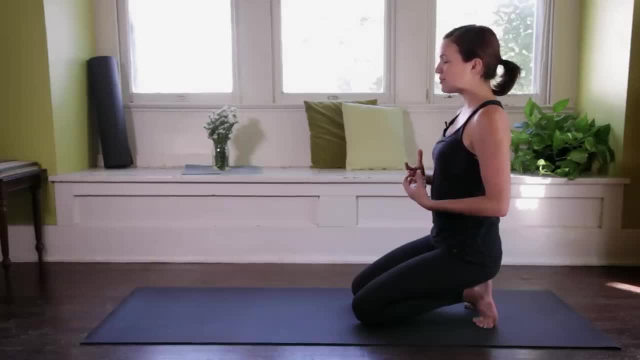 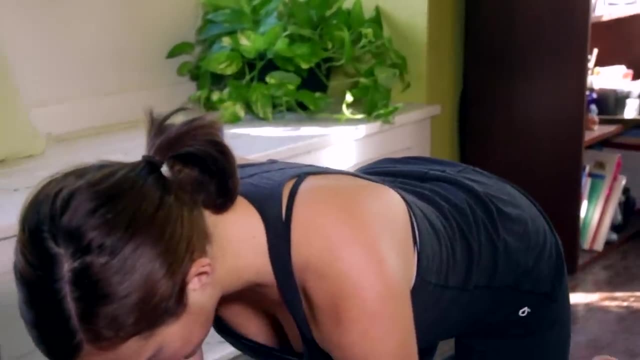 Stay connecting to that breath. Don't worry about how to breathe here, Just continue to play with the breath. Deepen the breath, Then we'll come back to all fours. Come onto the tops of the feet again. Inhale. Extend the right toes out long. 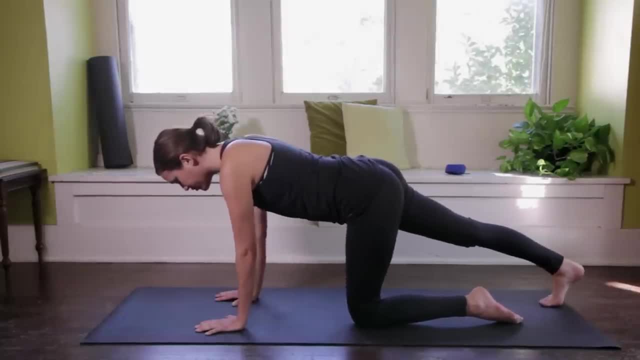 Go ahead and bring the right toes to the earth. We're just going to take a couple seconds here to breathe into the back of that right leg, Breathe into the calf. Notice, I'm not collapsing into my shoulders here, but I'm maintaining that lift so that 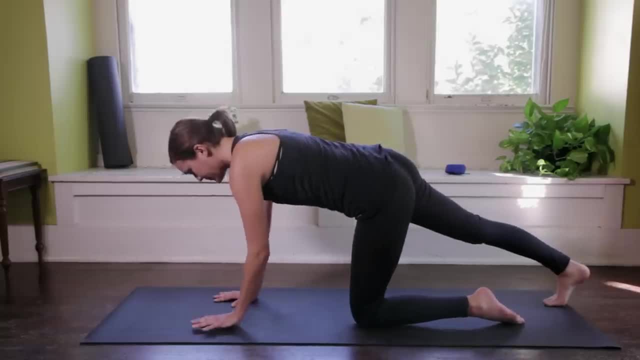 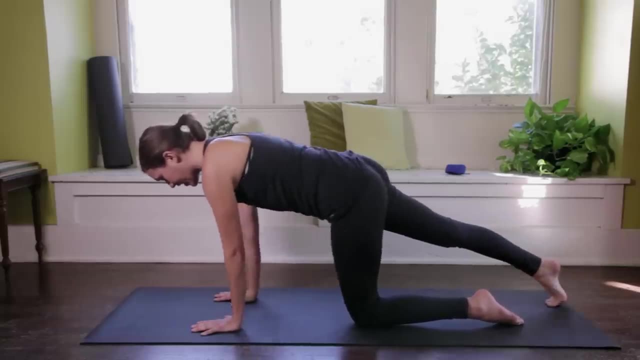 slowly I can begin to build that strength in the arms and just that energetic body, that lift. We call it hasta bonda, the hand to earth connection, this upward current of energy. Great, Notice how I'm rocking a little bit back and forth here, just finding that sit bone to. 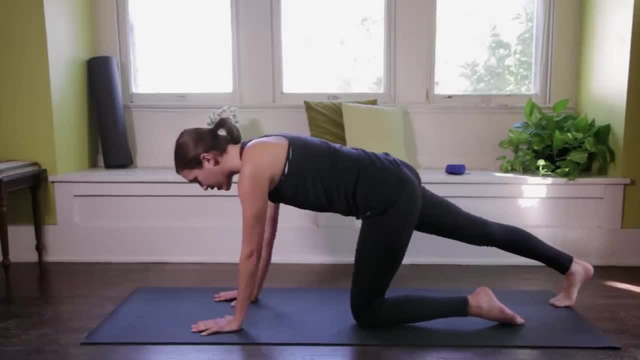 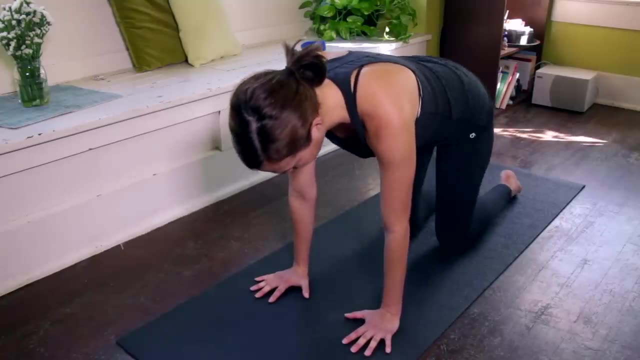 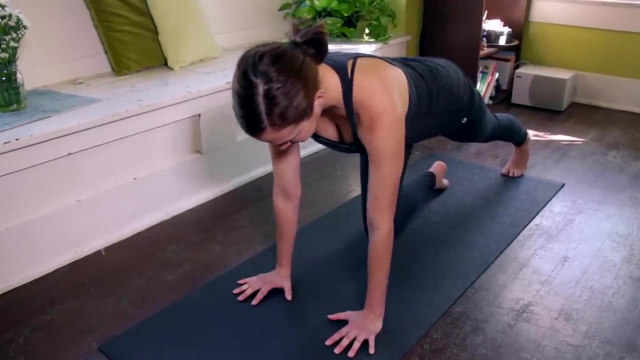 heel connection. I'm working at drawing my navel up towards my spine, Kind of knitting the lower rib cage in and keeping the neck nice and long, Then release back to tabletop position and take it to the other side, Curling the left toes under, now stretching out the back of that leg, the calf, while. 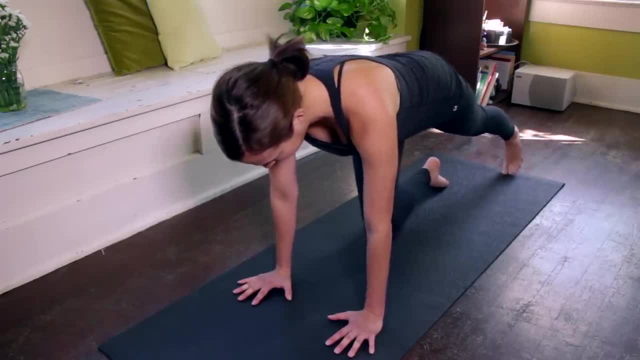 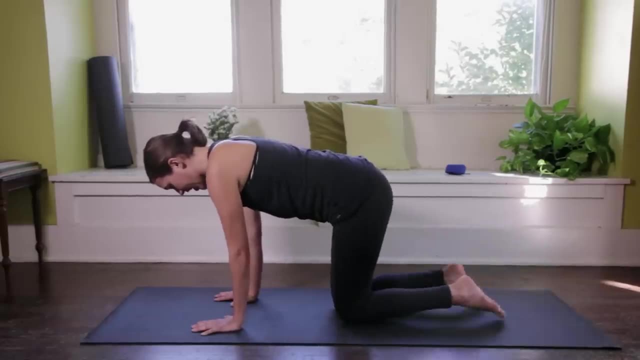 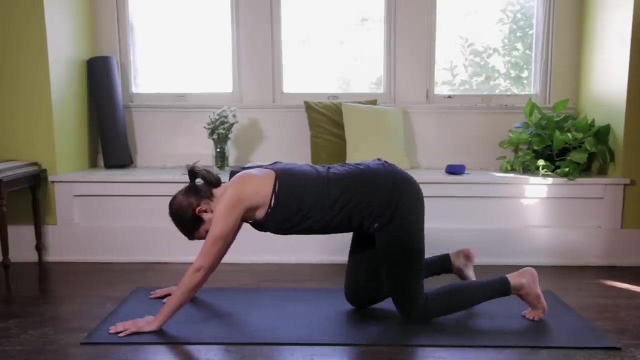 still maintaining a nice line from the crown of the head to the tip of the tail. Breathe, and then we'll bring it back to tabletop position. Great, Curl the toes under, Walk your palms out And then, slowly, We're going to walk the knees back here. 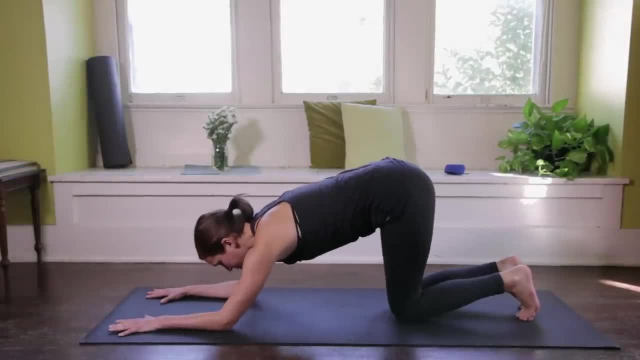 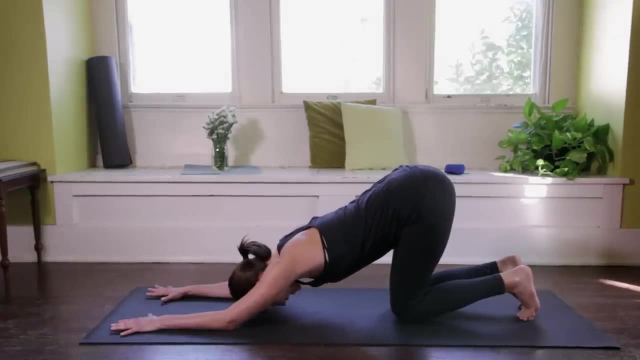 Elbows are going to drop in line with the shoulders and in line with the wrists, Then my pelvis is going to tilt up as my forehead maybe comes to the mat here and heart melts down towards the knees. Now, if your shoulders are having a wake up call right now, maybe you pulse in and out. 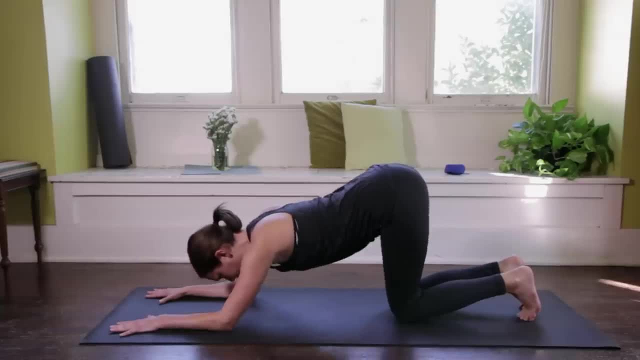 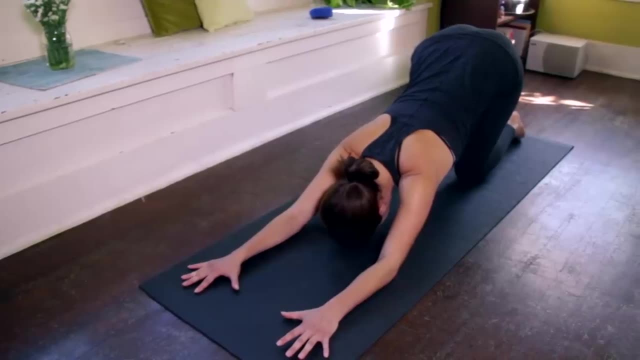 of it a couple times. We call this anahata asana or heart to earth pose. This is like a puppy posture here, Like a half downward dog. Good, Good, Good, Take a couple breaths here. sway a little from side to side. 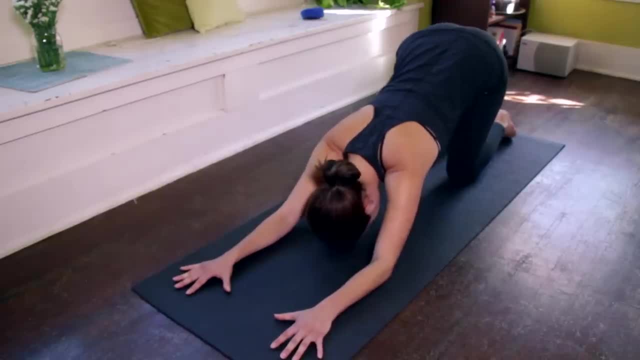 My shoulders are actually pretty tight, a little sore from practice yesterday, so I'm finding a little bit of movement. I'm never sitting in any sharp pain ever, but using my breath as a tool to move beyond the pain and find some movement. 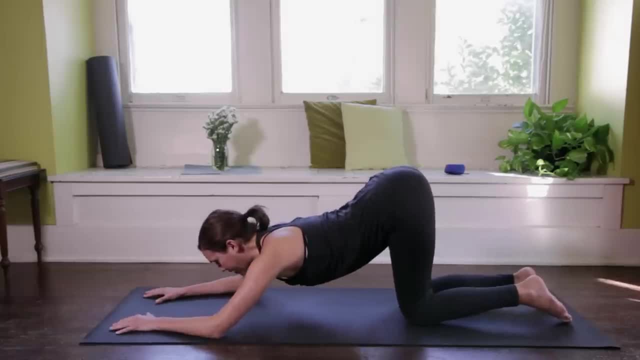 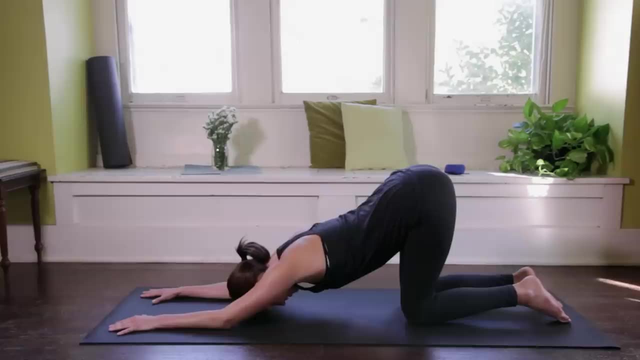 Again. notice how the elbows- they're going to want to come out here. See if you can keep them in line with the wrists and the shoulders. One more breath here, Heart to earth, Pelvis tilting up towards the sky. Good. 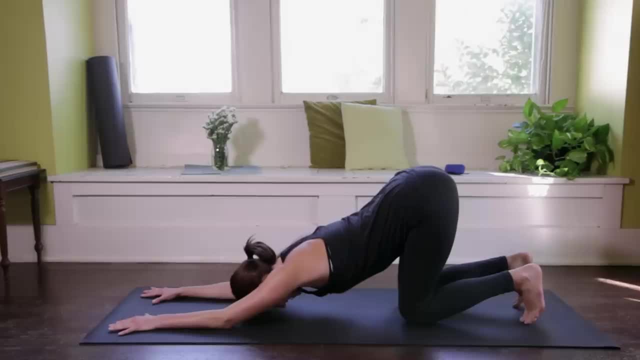 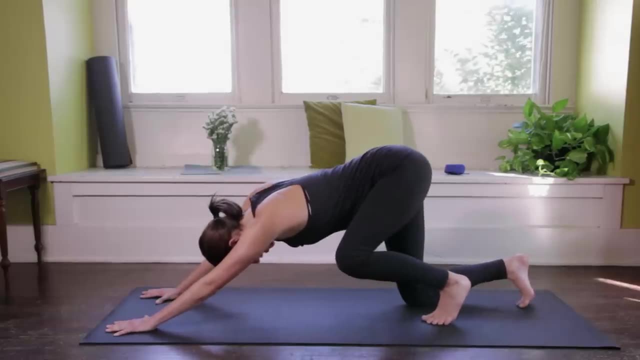 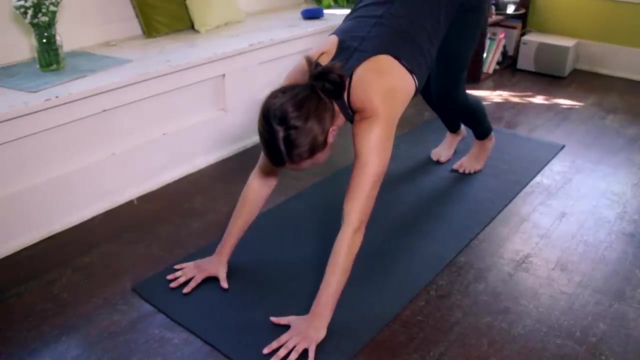 And then I'll begin to curl the toes, inflate at the heart, inhale, lift the heart, press into the palms and then, slowly, one leg at a time, nice and slow, I'm going to lift the sit bones up, dropping the left heel, then the right, and come into our first downward. 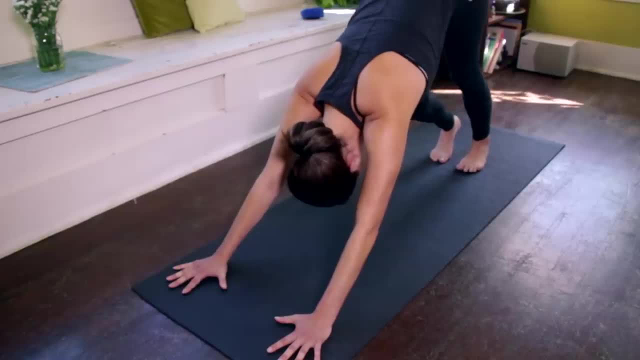 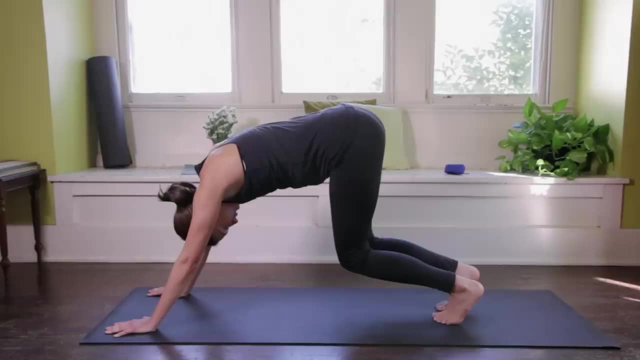 dog together Now, palms pressing like starfish into the earth, keeping that upward energy, that upward current up through the palms, through the arms. so I'm not collapsing my weight here. I'm finding this nice length in the spine and notice how I have really yet to straighten. 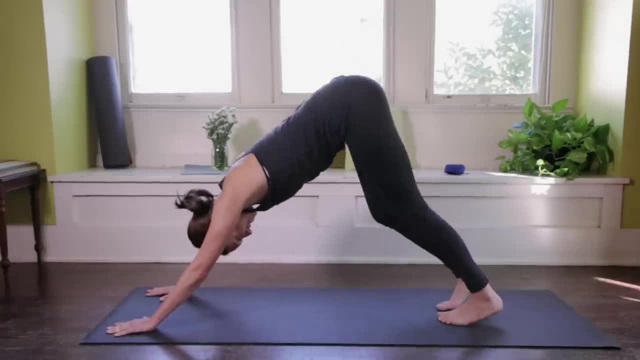 both my legs yet, So don't worry about what you think downward dog is supposed to look like. but my beginner's tip- and this is great for all yogis: we kind of always try to inspire each other in the yoga world. to come back to the beginner's mind, and I think downward dog is a great: 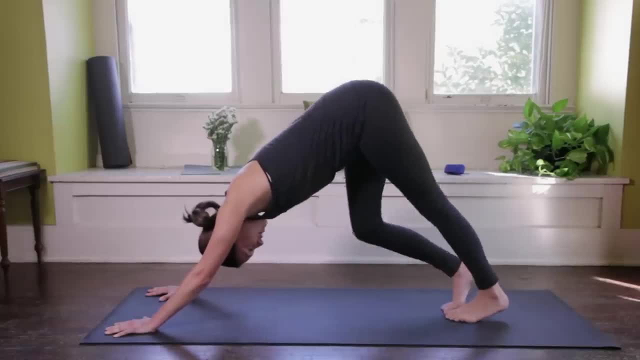 place to kind of check in with that beginner's mind by first maybe finding a little movement, pedaling the feet, drawing the shoulder blades in and together Take a deep breath in and then exhale, come back to the knees and walking the fingertips. 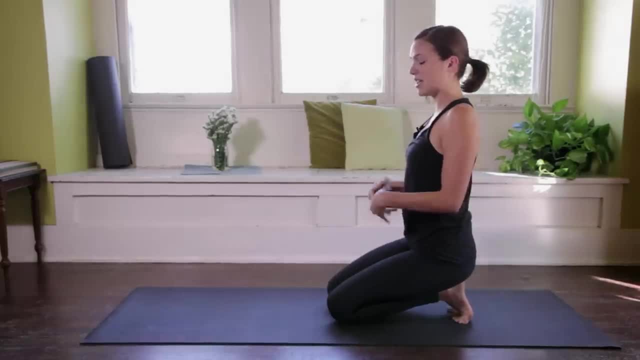 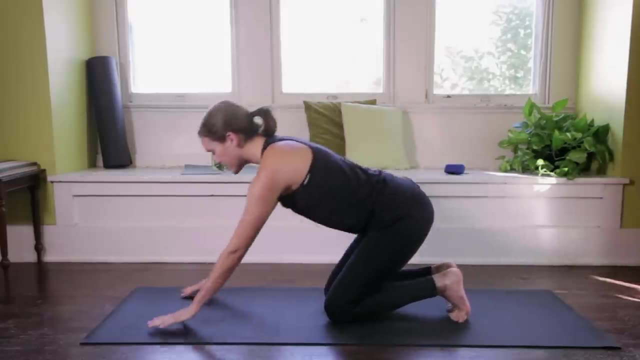 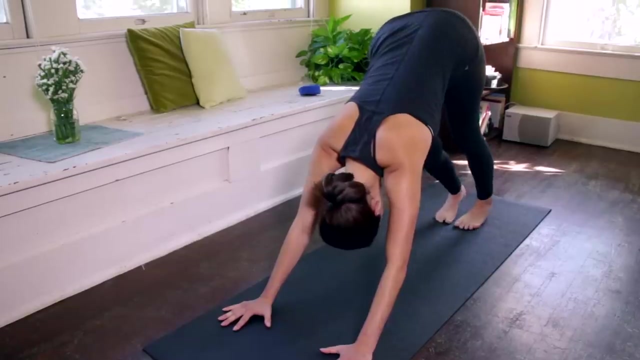 back up for a little rest, Loop the shoulders, maybe a couple circles with the wrists and we dive in for more. Here we go, Palms to the earth, belly to the tops of the thighs this time, slowly, slowly building to a nice still dog where we take a second here to be with the breath. 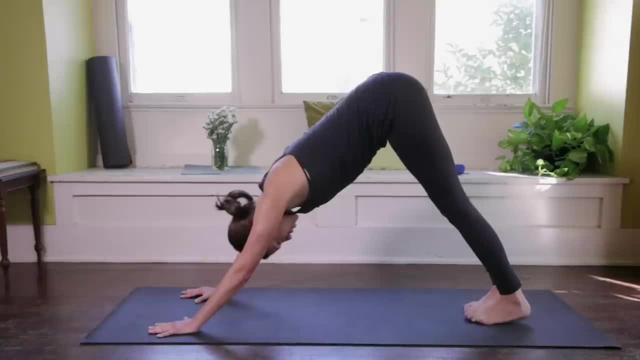 Now tops of the shoulders are drawing away from the ears. My two big toes are turned in just slightly, sit bones shining up towards the sky. I knit my lower rib cage together. I press up and out of my palms. I make sure my head 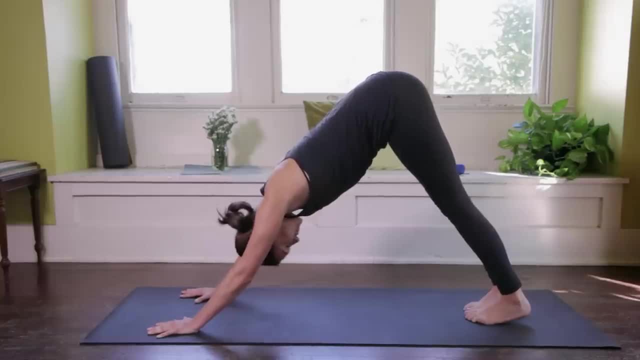 is nice and loose, not holding in the neck Tops of the thighs, have this sweet inner spiral going in towards the back of the mat. I take a nice deep breath in through the nose and exhale out through the mouth. It's allergy season here in Austin. 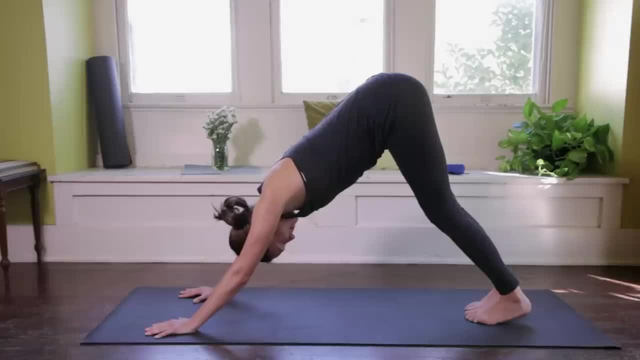 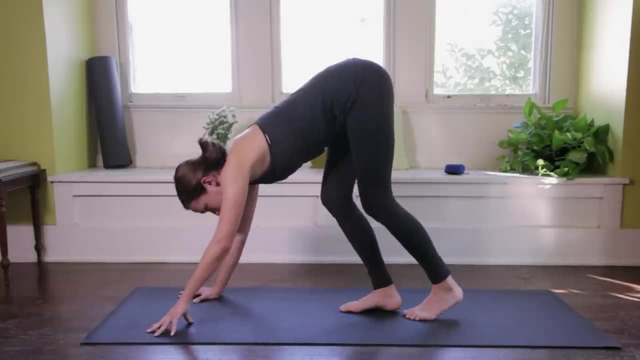 Inhale in through the nose And exhale out through the mouth. Bend your knees generously, Go for a little walk slowly up towards the front edge of your mat, Come on to the fingertips when you need to, and together we'll land in a forward fold. 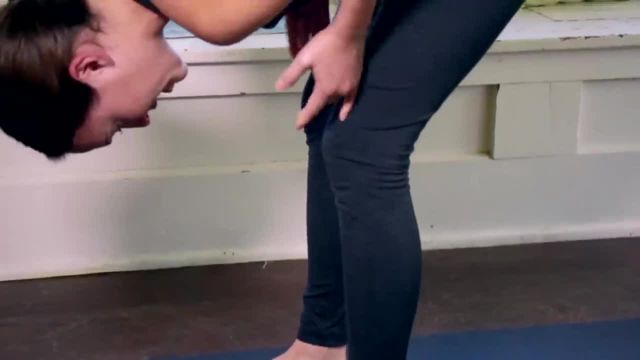 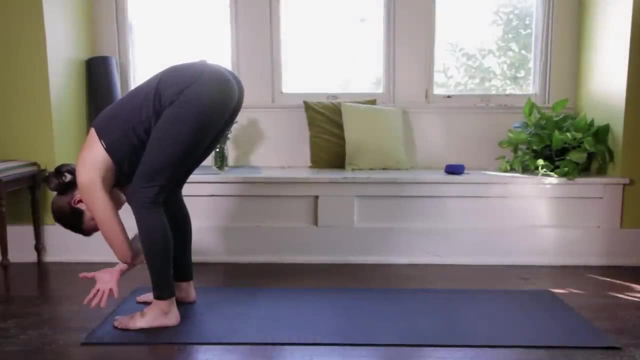 Feet, hip width apart, knees bent as generously as you need, and we let it all hang, breathe, Breathing into the lower back. Uttanasana: here We might grab the elbows and rock a little side to side, Then releasing the arms. 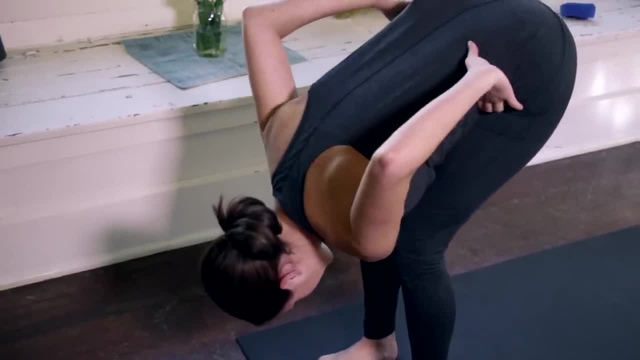 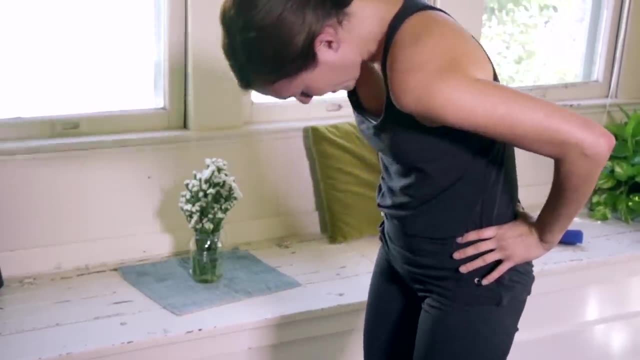 Bringing them to the waistline here, perhaps using the thumbs here to kind of hook behind the back. as I loop the shoulders, press in all four corners of the feet and slowly rise up, Coming into kind of a superhero pose here as I loop the shoulders, find that lift in. 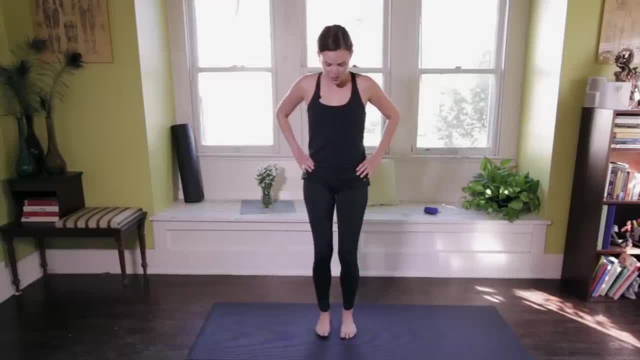 the chest And I'm actually going to move to the front here so you can see me a little bit better. So I'm coming into a mountain pose- We call this Tadasana- with the feet hip width apart. toes are pointing forward and really. 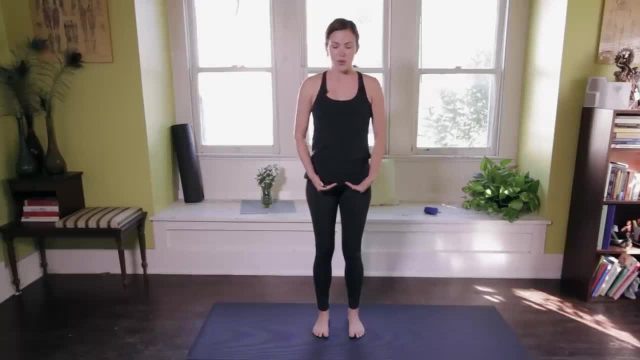 this is about connecting to the earth, feeling strong. We practice this here so that later on, when we come into all these kind of other fun, crazy poses, we've practiced again that upward current of motion while also grounding down. So for now, just check in with the feet spreading awareness through all four corners of the 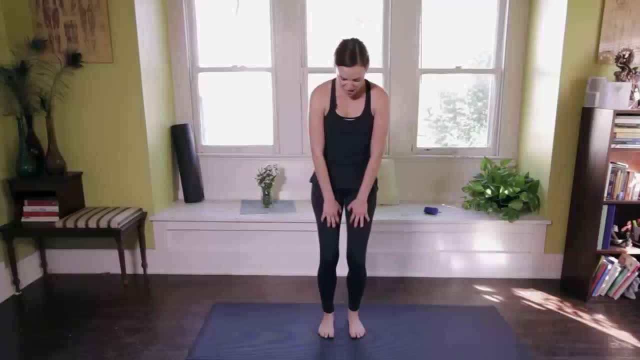 feet, perhaps drawing energy up through the arches of the feet, maybe even lifting the kneecaps, toning the quads, just kind of bringing a little active energy into the body as once again we draw the palms together at the heart. 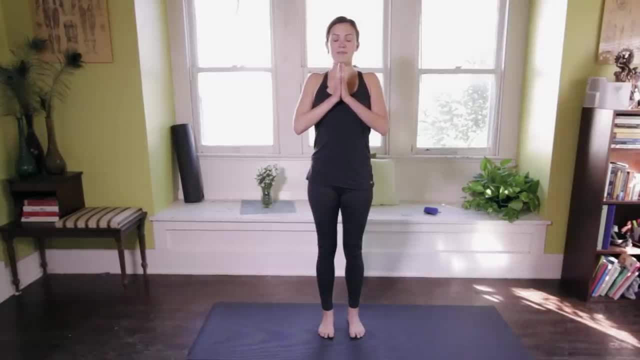 And aha, Lift the sternum to the ground, Good, Good. Lift the sternum to the thumbs. Tuck your pelvis in everyone And again, close your eyes. find that head over heart, heart over pelvis- this time pelvis. 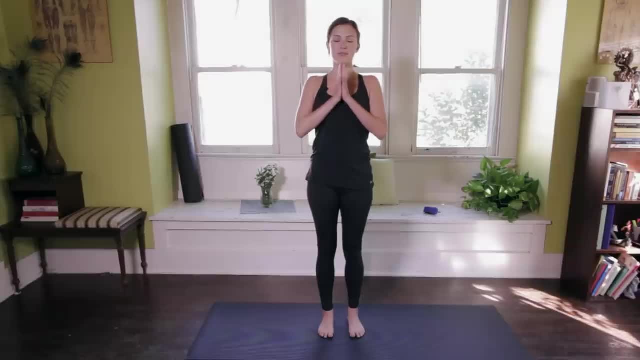 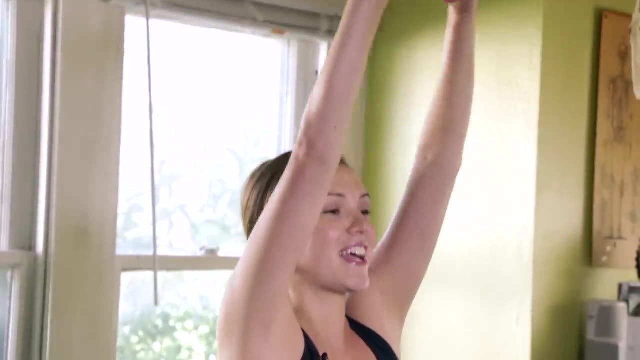 over heels or the center of the heels. Interlace the fingertips, soften the knees, find a little buoyancy here. as we inhale, Reach forward up and back- Nice tall stretch here- and then exhale, releasing the fingertips down, just like we did when. 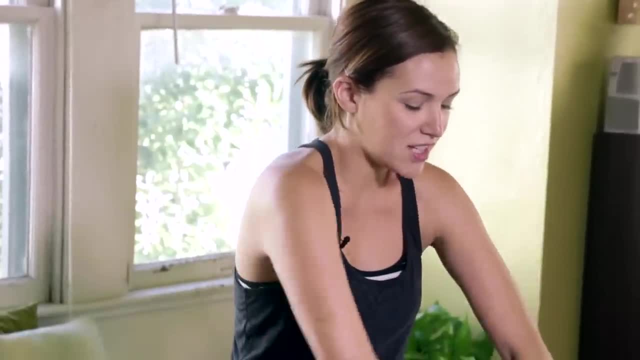 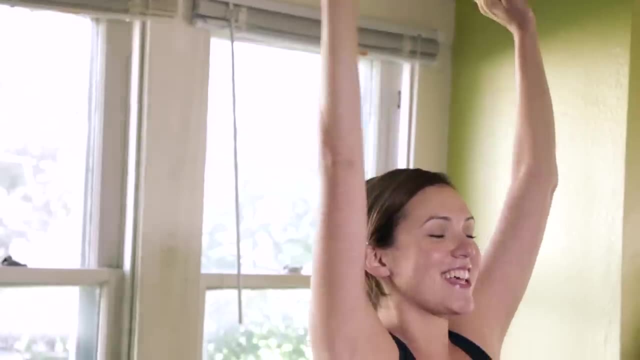 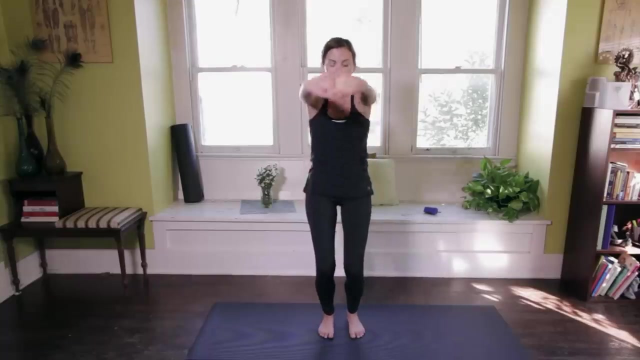 we were seated, opening the chest. Soft knees reaching forward, up and back. Tailbone lengthens down. tuck your pelvis and exhale, opening the shoulders. fingertips might move a little bit here, maybe checking in with the neck this time. inhale forward. 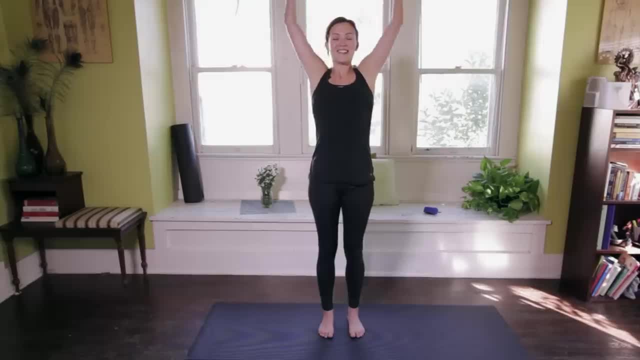 up and back, lengthening the tailbone down. exhale, Ooh, awesome. Take a second here to draw a couple circles with your nose. Check in with the neck. Good, Good, Good. Often we think in yoga, you know we have to be in these crazy pretzel shapes, but really, 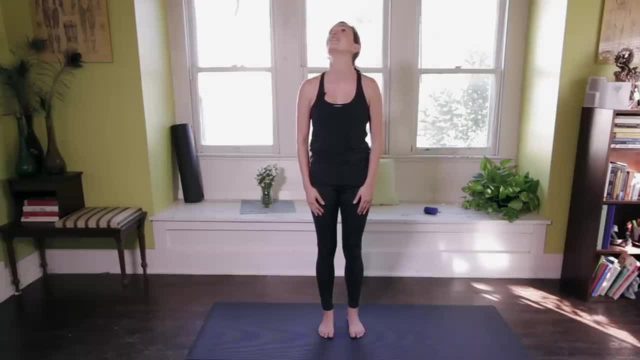 for me each day. yoga really begins with this movement, this gesture, drawing circles one way and then the other. checking with my neck, grounding down through my shoulders and elbows and fingertips, Feels good. Okay, take a second soft knees to bend the knees and then reach the fingertips up- Volcano. 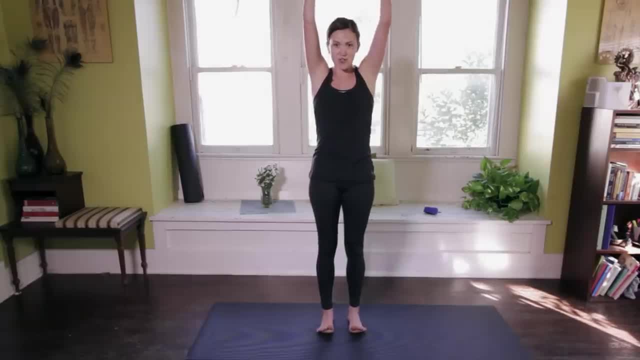 Pose. I'm lifting my toes here just to press into all four corners of my feet. I'm tucking my pelvis in. The arms might get tired right away here. With practice you'll notice this gets easier. Pull the thumbs back. 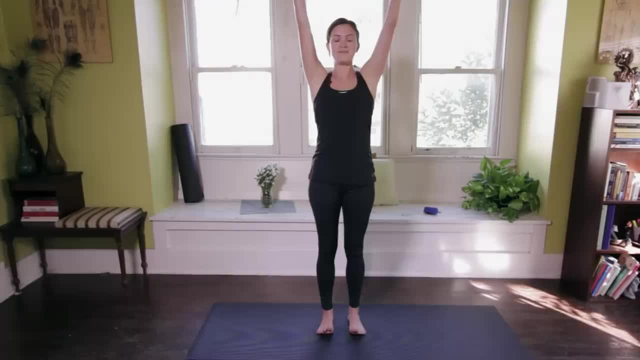 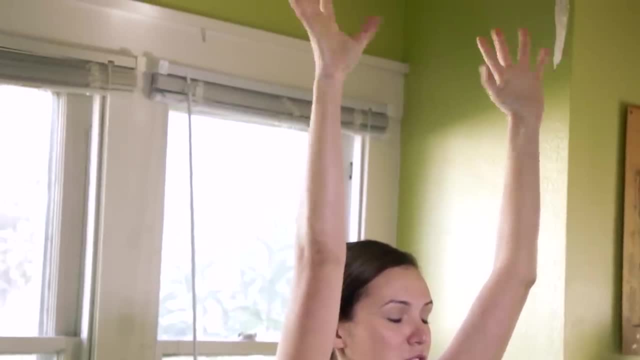 Find a flying V. if you feel like this, like no space, Find some space. Release the toes back down, if you haven't already, and breathe. Spread the fingertips in celebration of you and your new yoga practice. Then take the right hand and grab the left wrist. 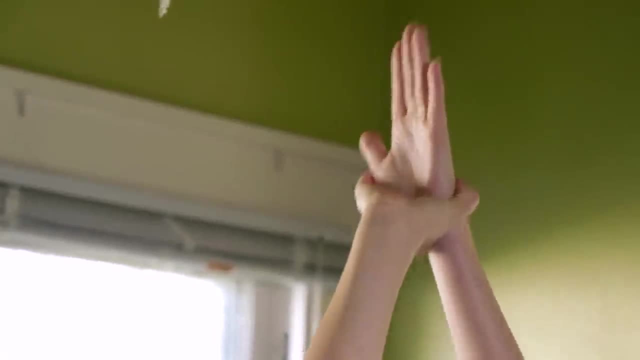 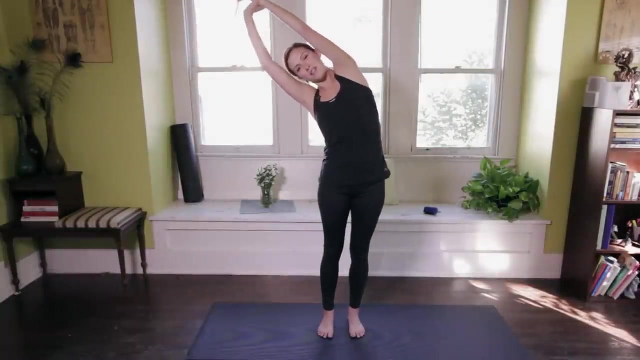 Again, just like we did before in the side body stretch, think up and over. so, rather than just to the side, yowch, Think up length, length, length and then over. This will look a little different for everyone. 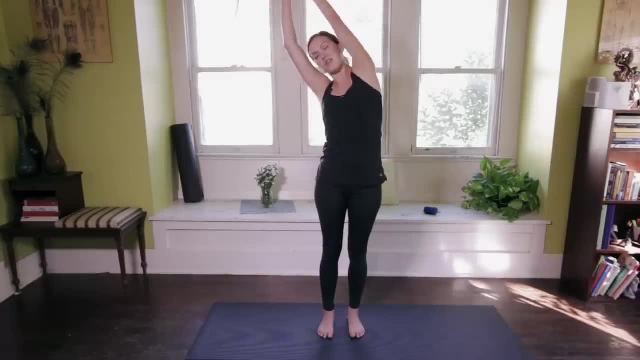 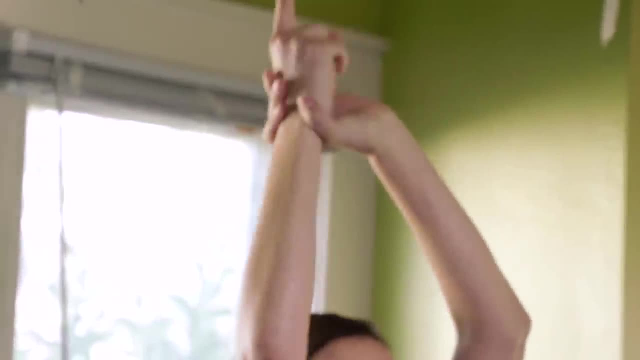 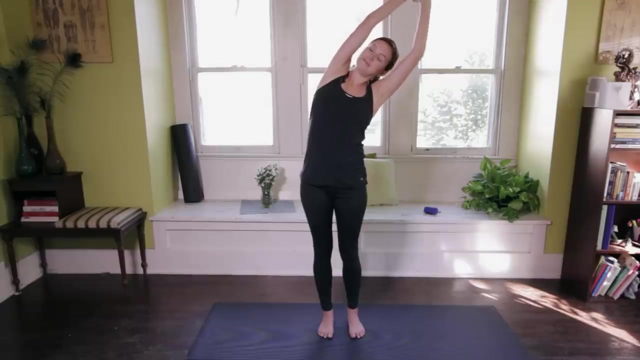 Again. you can find a little self-expression here, as you maybe sway a little back and forth And then we'll come back to center. I know arms might be getting tired here. Hang with me, Grab the opposite wrist, Think up and over as you breathe into the stretch. 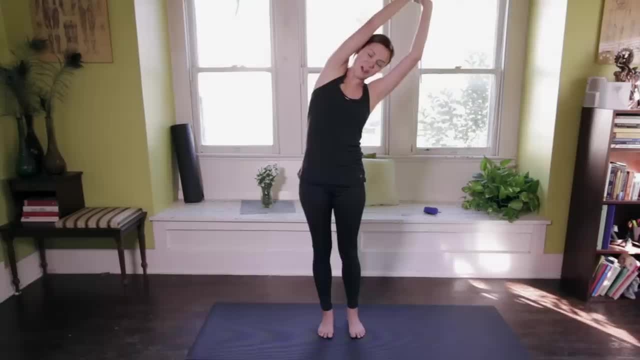 Ground down through your feet. Remember that sit bone to heel connection, Tuck your pelvis And then we come back to Volcano. Pose for one breath. as we inhale, Look up by drawing a line with the nose up and then exhale back down at the heart. 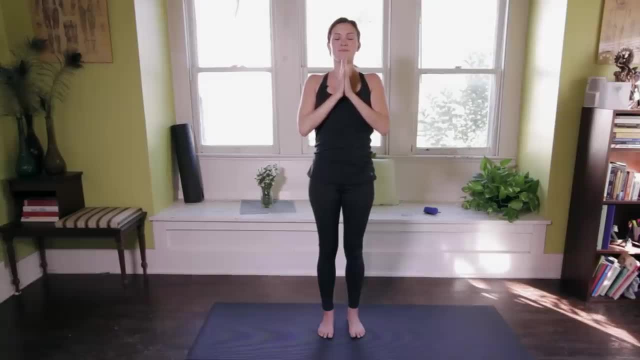 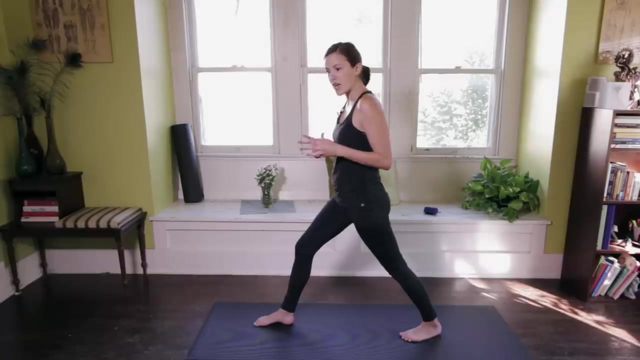 Palms to the sternum as we lift it up. Awesome, Bring the hands to the waistline. So we're going to take the right foot forward and the left foot back. I'm wanting to get to a place. I'm not going to spend too much time on all the fine details. 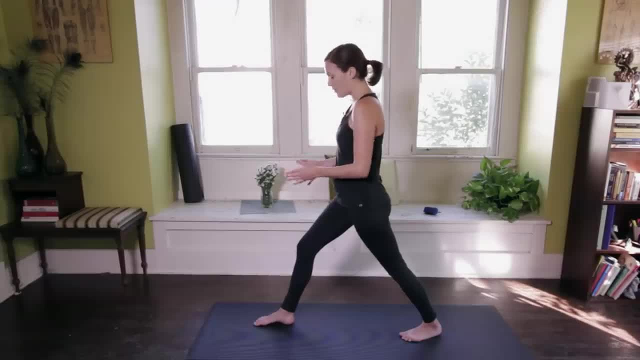 because I'm wanting just to just get a taste for things. So right toes are going to point forward, Left toes are going to point forward, Right toes are going to point towards the front left corner of the mat And I'm going to make sure that I'm on two planes rather than one tight rope like two. 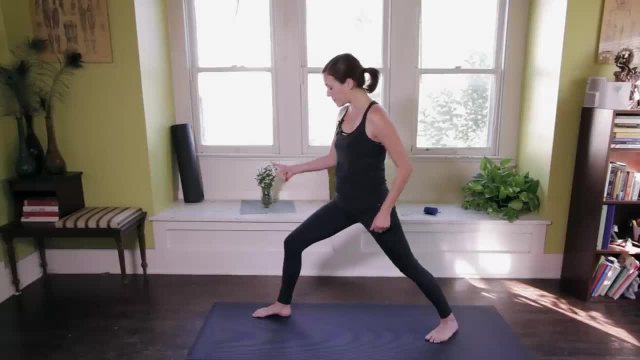 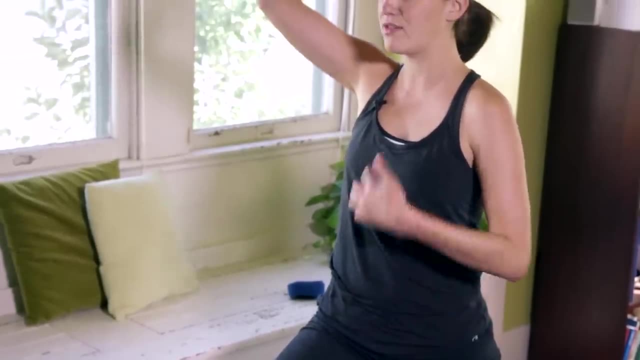 skis. So I have lots of space like maybe hip point apart, Take your right thumb, pull your right hip point back, then see if you can tuck your pelvis and do this thing. we've been working on where we align head over heart, heart over. 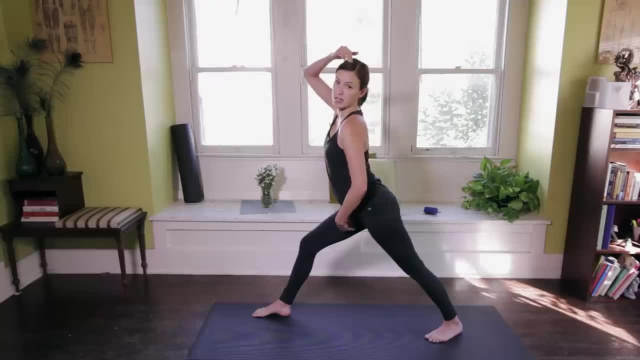 pelvis. Now the tendency is that the pelvis is going to want to spill back hey-oh. but I'm going to lengthen the tailbone down, tuck my pelvis and find integrity in the torso- kind of lighting. 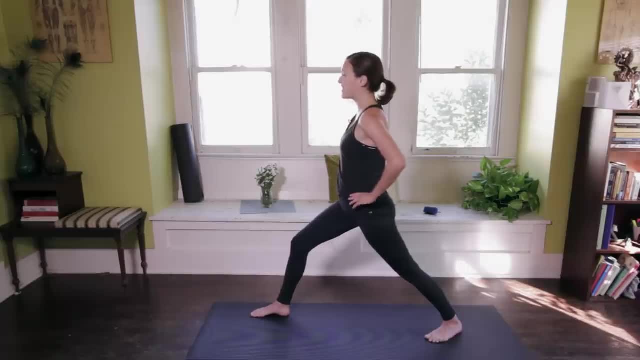 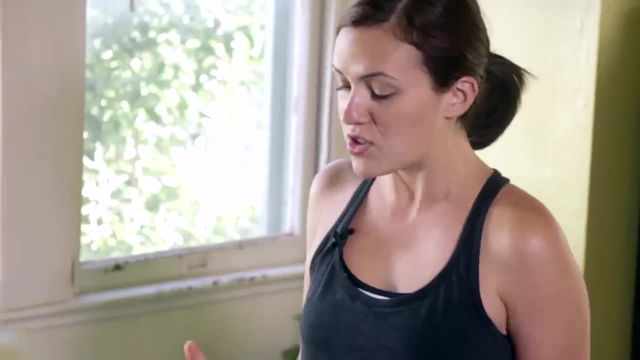 that fire in my belly. Great Hands on the waistline here as I loop the shoulders and breathe. Back heel is on the earth strong. Both legs are charged by maybe squeezing the inner thighs together, finding that scissor effect. Got excited there. 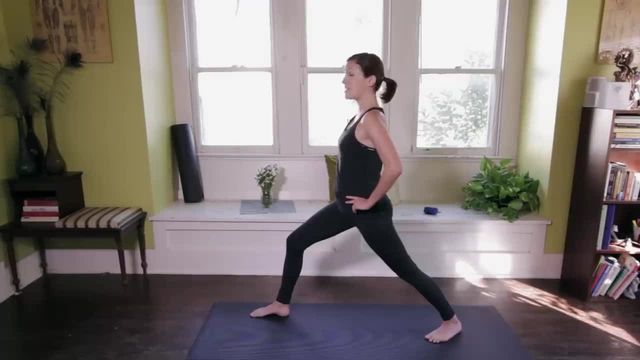 And then finding that length in the crown. Breathe here. You can stay here bending that front knee generously. Eventually I'm going to want to get to a place where the bottom of that thigh is parallel to the earth, but in due time, in due time. 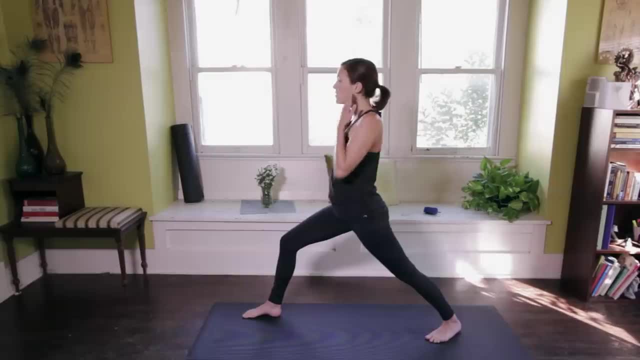 So I can stay here Hands on the waist, or I can reach the fingertips behind the ears and reach it up. Voila, I'm in. warrior one, Virabhadrasana one. Pull the thumbs back. Remember your alignment. Draw your navel in slightly. 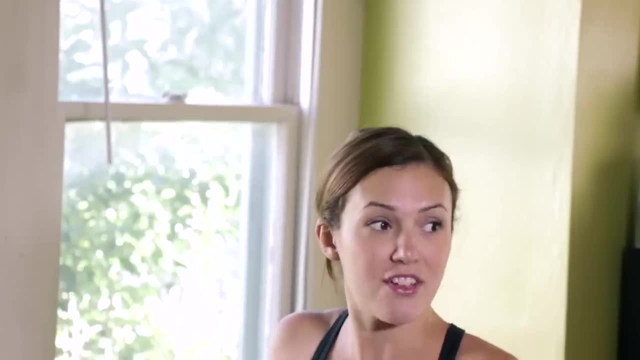 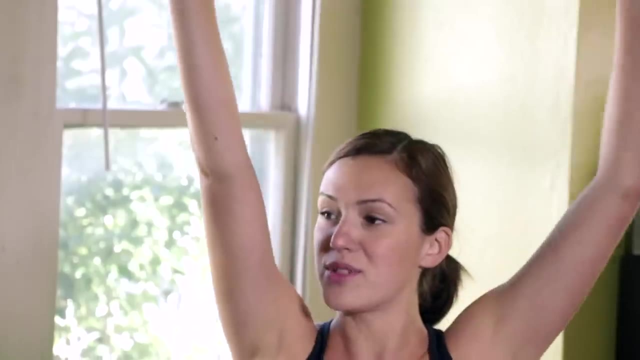 Breathe here If you feel like whoa, hug those inner thighs together, Find stability as you breathe, Take a deep breath in, Inhale As you exhale, open up towards the left side of your mat. Ah, warrior two. 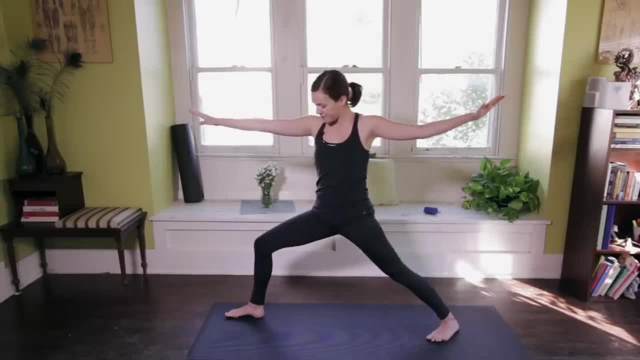 I might walk my front toes towards the front edge of the mat And I might find a little bit. I might find a little bit more space here. a little wider stance is what I'm trying to say as I pull my pinkies back and find that lift in the heart. 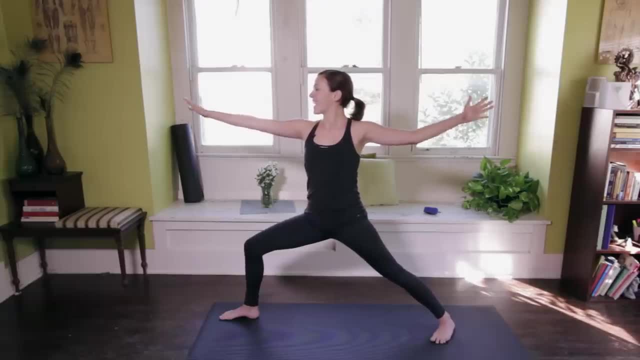 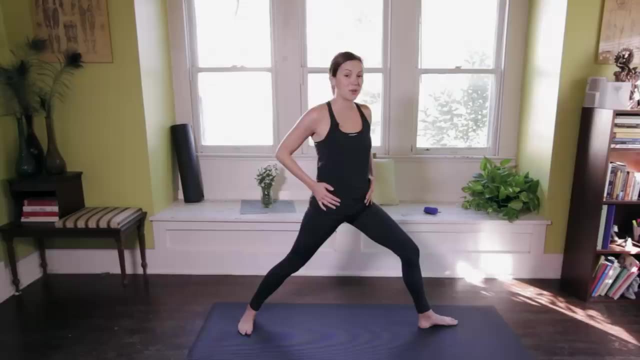 Breathe here Strong legs And then exhale hands to the waistline and I'm going to turn my right toes in and my left toes out to take it to the other side. Now we're going to work in reverse order here. so a little yoga for the brain, too, coming. 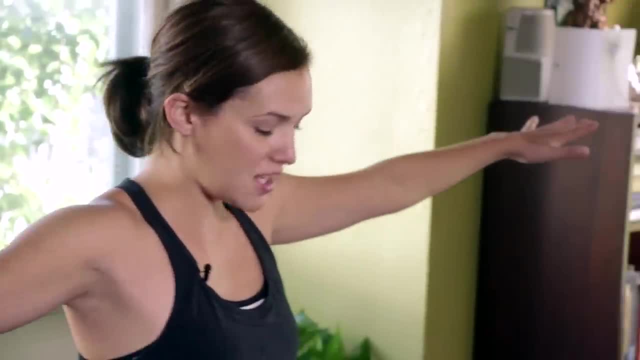 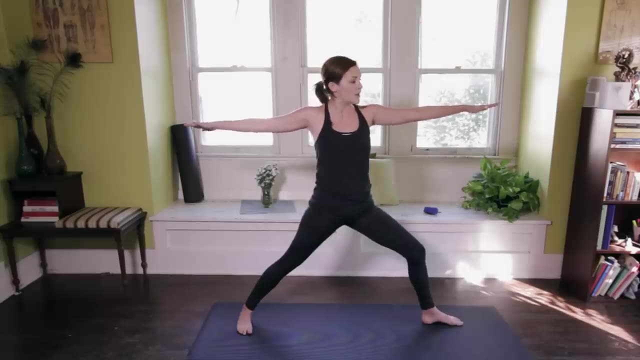 into our warrior. two on the left side first Bend the knee. The tendency is you're going to be like I'm not strong So I'm going to hang out. I'm going to like not bend that knee so far, right away, but I think you'd be surprised. 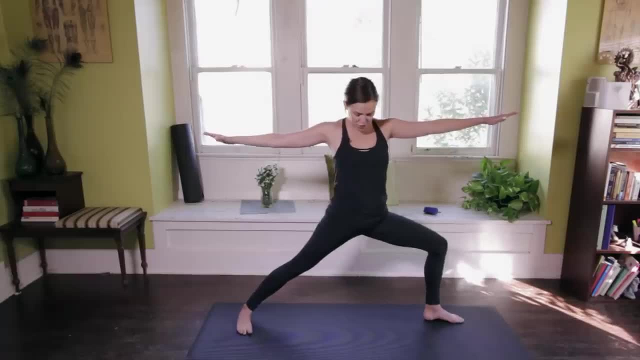 Get in there, Get a little juicy, Make sure your feet are stacked just where you need them so we're not on that tight rope. We're really paying attention to our foundation, working our yoga poses from the ground up. Deep breath in here and exhale hands to the waistline. 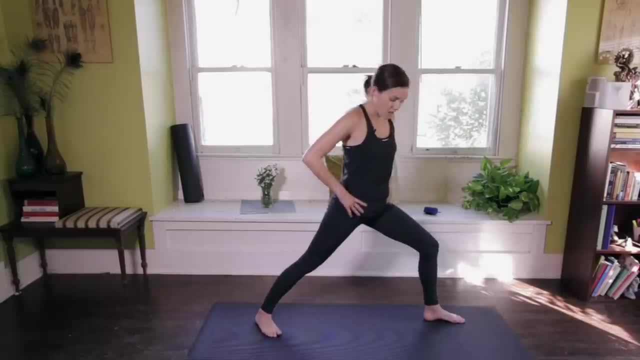 Then I'm going to step the back foot in just a little bit so that I can bring that back heel to the earth. Strong legs, Strong lower body. As I move, my hip points gently towards the back edge, which is now the front edge of 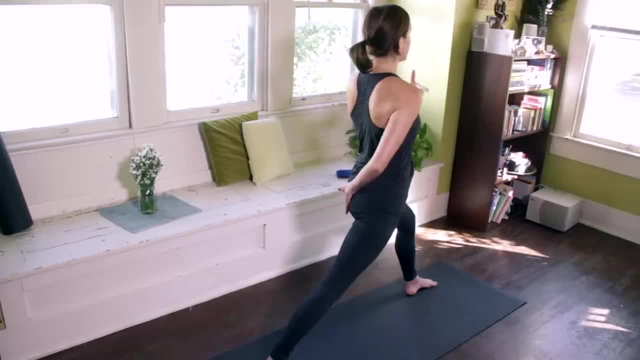 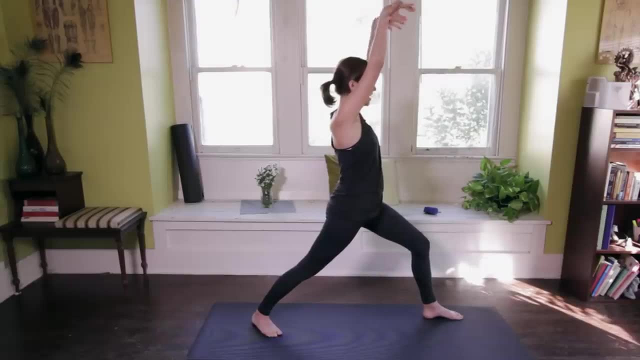 the mat, lengthen the tailbone down, Find that lift in the heart. We can stay here or we can reach the fingertips behind the ears to come up, Voila warrior one on the opposite side. Again, don't worry about trying to create that perfect image, that perfect asana. 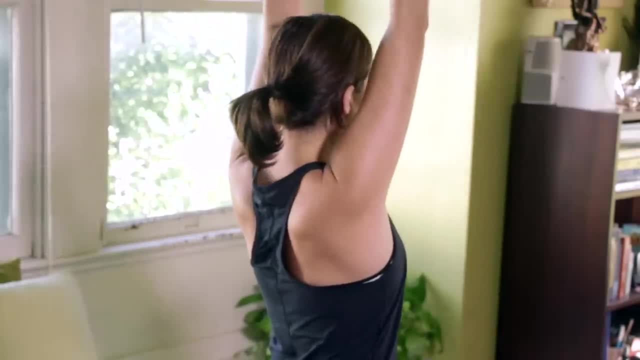 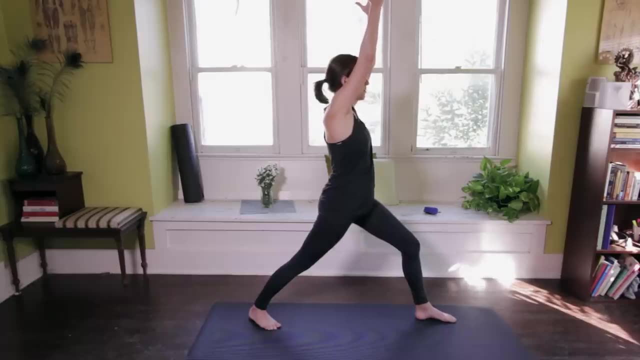 It really is about having an experience and then growing the pose. It makes it fun too and less work. Okay, I slung Inhale in here. Hang with me, Hug those inner thighs towards the midline and, on an exhale, float the fingertips down. 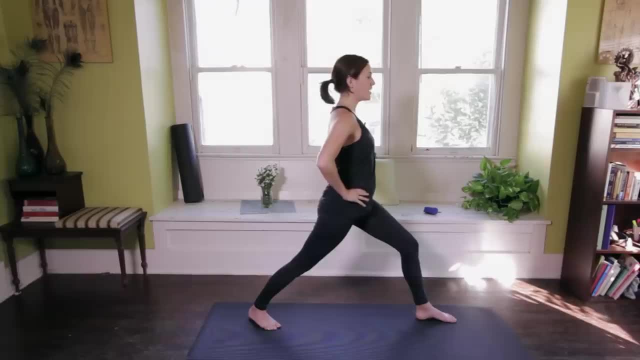 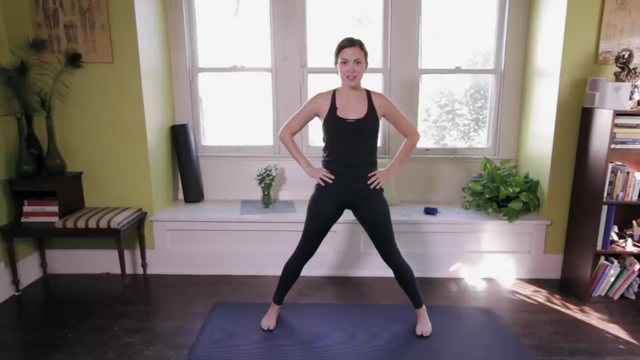 back to the waistline for a little stability, hooking my thumbs behind here. Then I'm going to turn the left toes in, come back to center and I'm going to heel-toe, heel-toe my feet back into center. 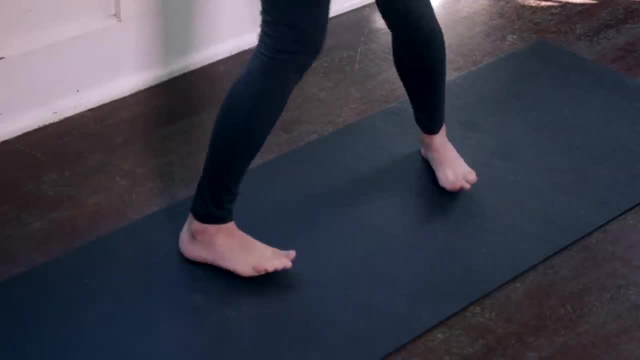 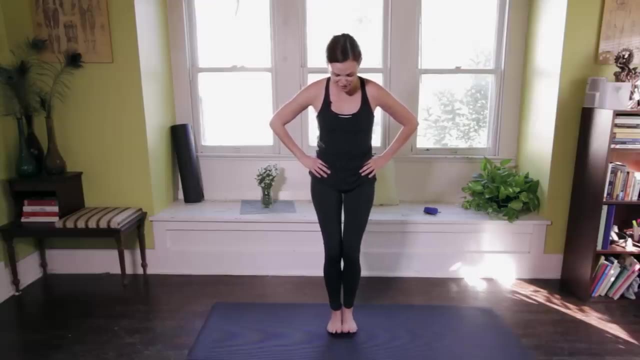 So when you hear that in yoga class, that's what this means: Heel-toe, heel-toe- It's kind of silly. Okay, This time I'm going to challenge my center of gravity by coming feet flush together, Okay. 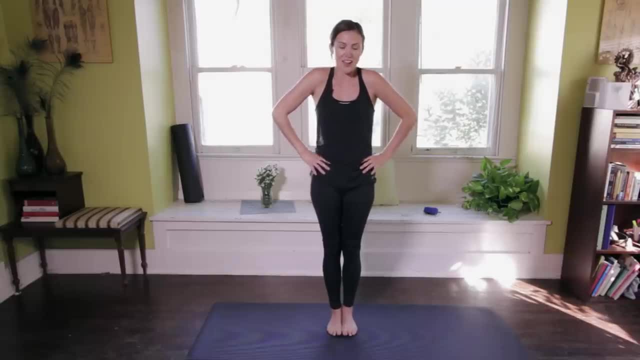 Before we were hip width apart. Now I'm going to stand up, nice and tall, in Tadasana where I'll finish my practice today, bringing the fingertips down, maybe closing the eyes, kind of challenging that center of gravity, taking the experience of my practice and drawing the palms together at the heart.